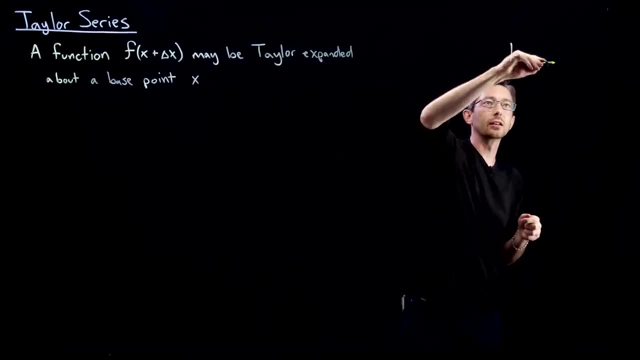 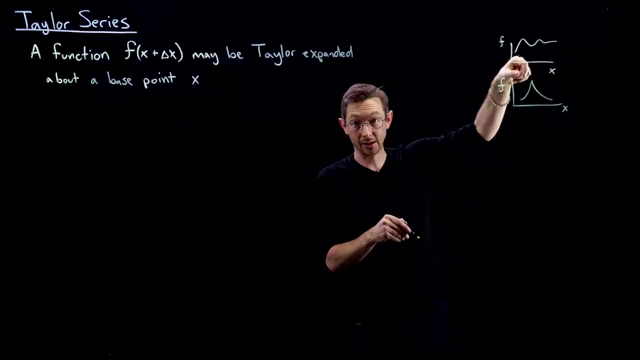 smooth, Like it's not. we're assuming that our function, you know, f of x is smooth and is not, you know, cuspy. Because if my function has a cusp or a discontinuity, then the derivatives are not going to exist or be matched at this point, And so this isn't going to work. So a function f can. 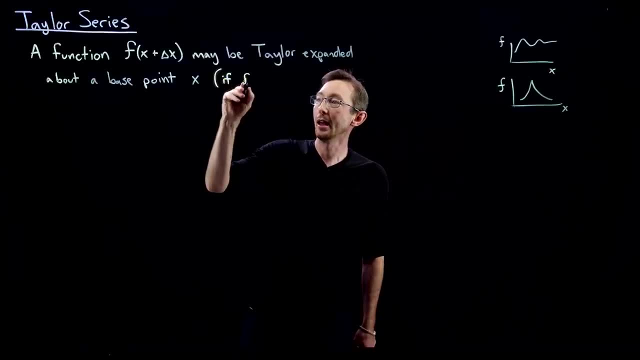 be? Taylor expanded about a base point. you know, if f is smooth at x, meaning all of its derivatives exist and are continuous, That's what smooth means to mathematicians. And specifically, we're going to say- I'm going to write this in pink- We're going to say that f of x plus delta x 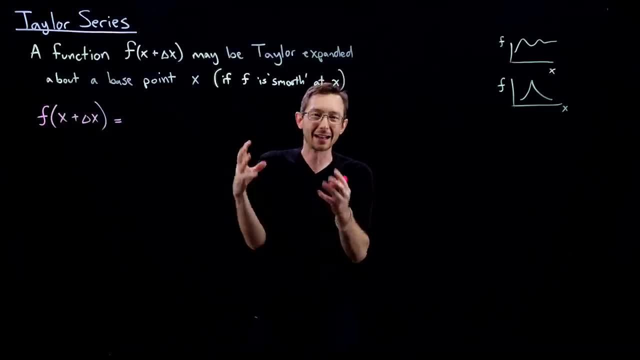 is going to equal. So we're kind of assuming that delta x is small. This doesn't have to be small. We could have large delta x, depending on the radius of convergence in the series I'm about to write out. But in my mind I often think of delta x as kind of close by. It's a small little. 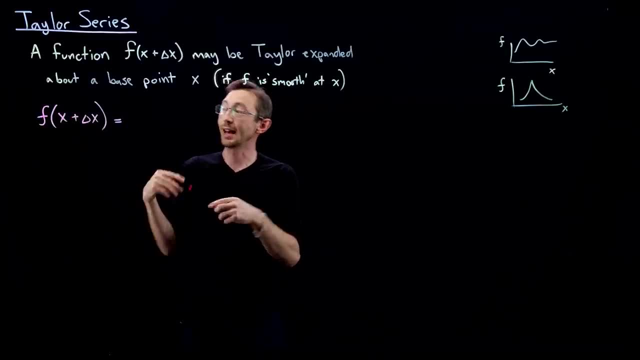 point close to x, And so So f of x plus delta x is first off. the first approximation to this would be that well, okay, it's just f of x, And then the next correction term would be plus df, dx. 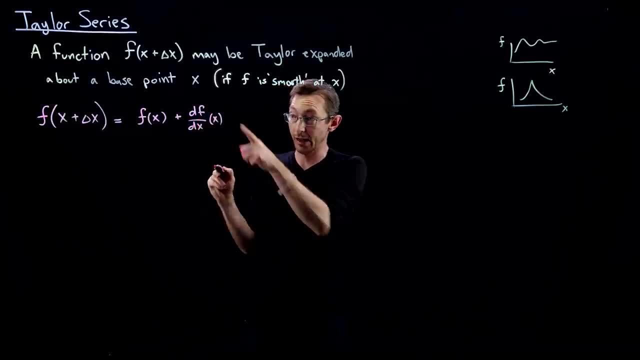 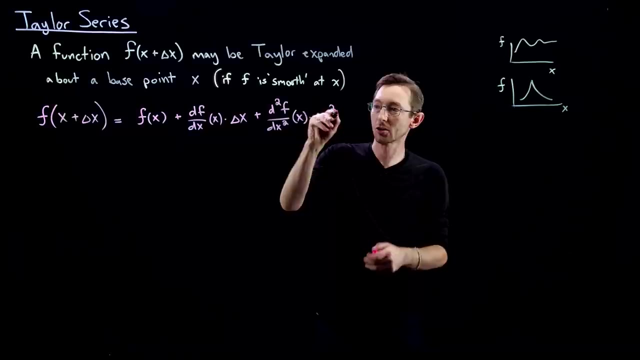 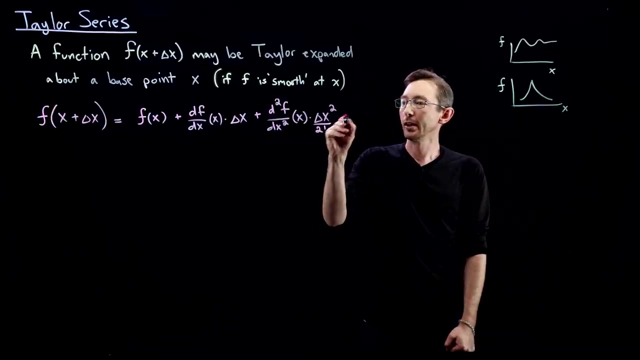 This is the derivative of f with respect to x, evaluated at my base point, x times delta x. Okay, this is my like first order correction, Plus the second derivative, d squared f dx squared evaluated at x times delta x squared, And this is going to be divided by 2 factorial plus d cubed f over dx cubed times delta x cubed over 3 factorial. 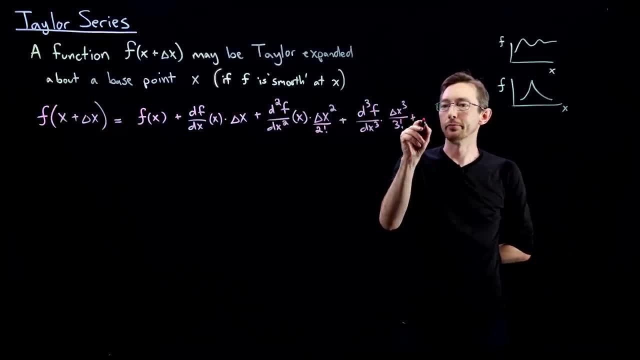 plus dot dot dot dot dot, forever and ever and ever, You know. plus dot dot dot, Plus d. the nth, The nth derivative of f with respect to x, delta x to the n over n factorial: plus dot dot dot. 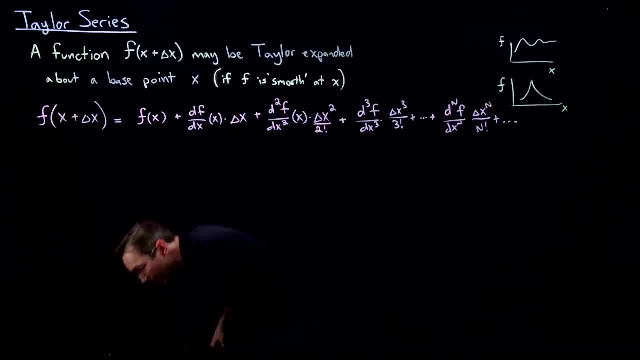 And this is going to go on forever and ever and ever. That's what the Taylor series does, is essentially- you know, this is an exact expression- If my function is smooth and all of its derivatives exist and are continuous at that base. point x. 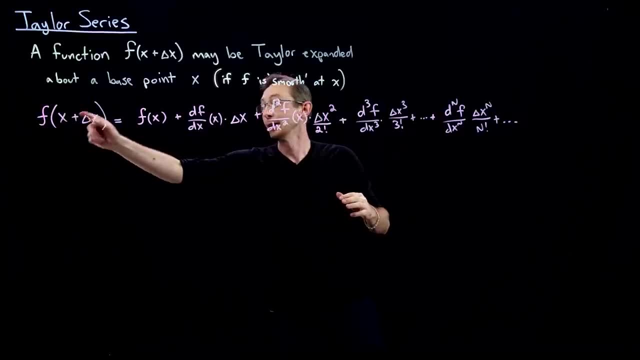 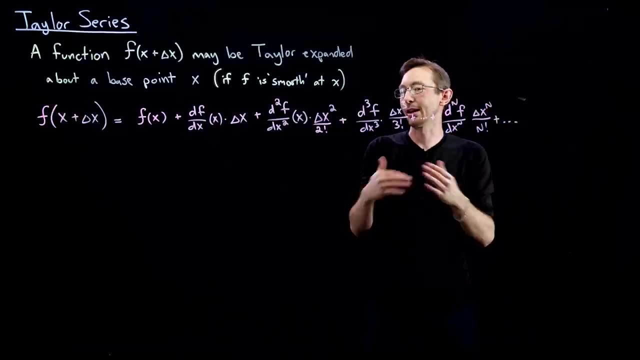 then I can basically expand out this function at nearby points in terms of this infinite sum of all of these derivatives. Now again, this is not all. This is a whole class on calculus, so I'm not going to go through all of the properties and derive this from scratch. 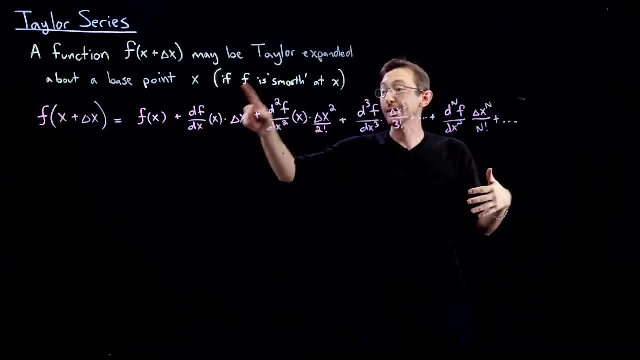 I'm showing you what it is, I'm reminding you what it is. We're going to actually plot this approximation for a function like sine of x or cosine of x in MATLAB and in Python, And again I you know kind of from a numerical perspective. I like to think about this often as delta x is a small perturbation for my base point x. 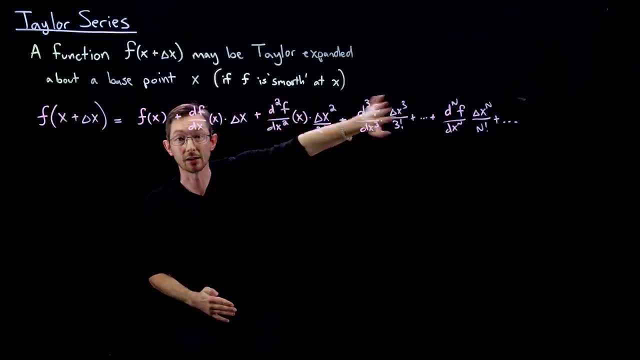 And so I might not want to actually compute all of these terms. I might want to chop this off. you know, at first order, At just you know, my linear delta x term, or at second order, at my first, you know, my delta x squared term. 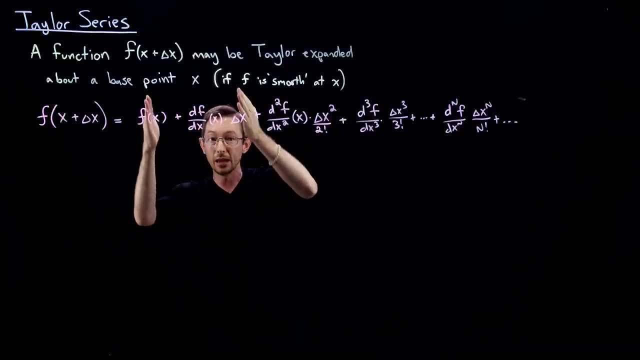 And I want to know how good that approximation is. if I chop this thing off, if I approximate this at some finite- you know, finite- expansion n, And so you'll see, if delta x is small, then each of these terms should get smaller and smaller and smaller, right? 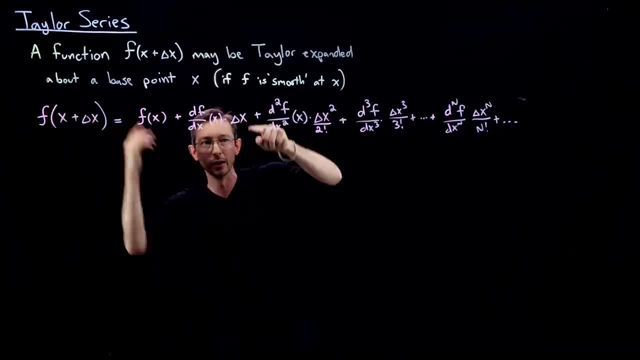 Like delta x squared is smaller than delta x. Let's say delta x is like 0.1. Then this is 0.01.. This is 0.001.. You know, these get smaller and smaller and smaller, And so this approximation should get better and better and better the more terms I add. 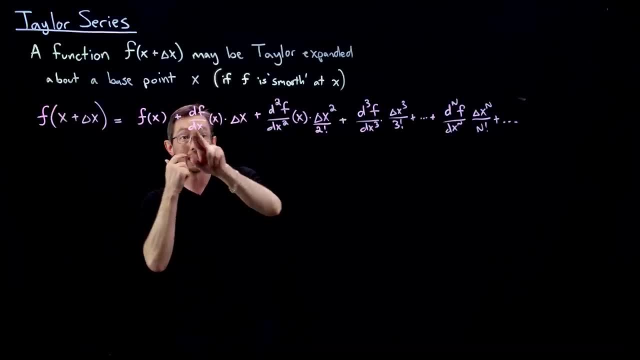 So, even numerically, if I want to approximate this function, I might only need to add up the first few terms in this series. But if I add up all of the terms, this is exactly true. This is the Taylor series expansion- okay. 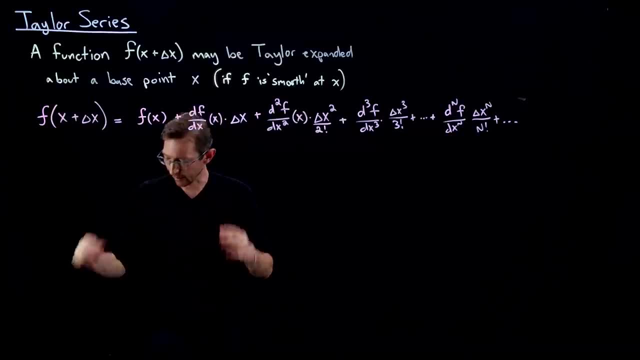 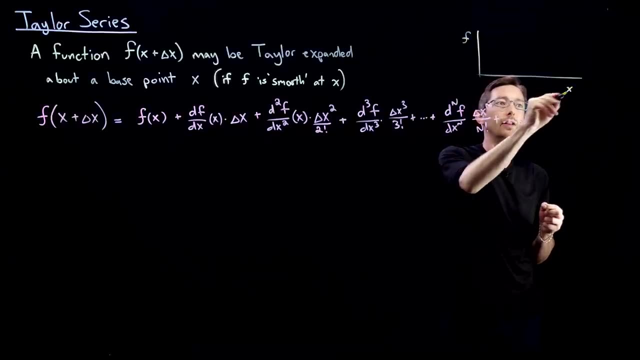 And this is in fact true for any delta x in a. maybe I'll draw a little picture of this. So again, you know, remember I was drawing this function f of x And I said it was continuous. Let's say this is my base, point x. 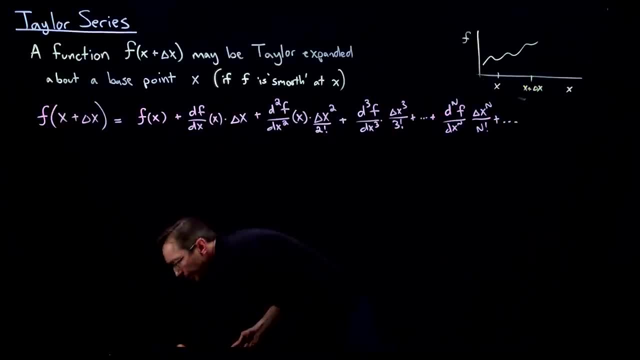 And this is x plus delta x, Then this Taylor series expansion is valid and it holds for any delta x until I hit a point where my derivatives are discontinuous. So this Taylor series expansion is valid for this large. we call this the radius of convergence. 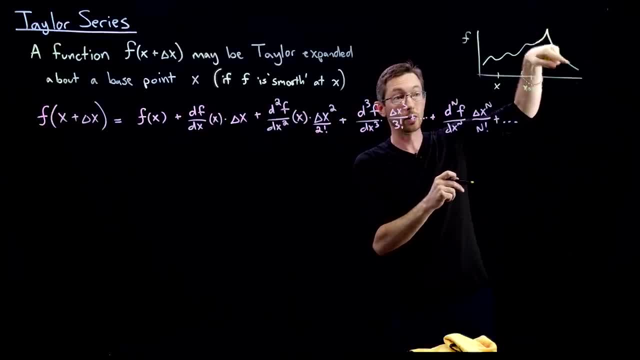 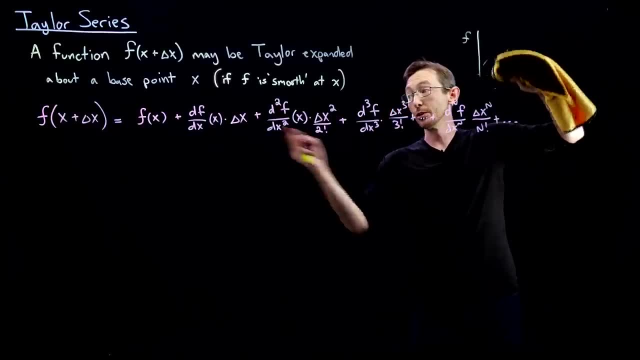 This will converge until I hit a discontinuity or a cusp or somewhere where these derivatives are not smooth and don't exist. So you can actually do this. So you can actually do this for big delta x, as long as you keep all of the infinite terms in this series. 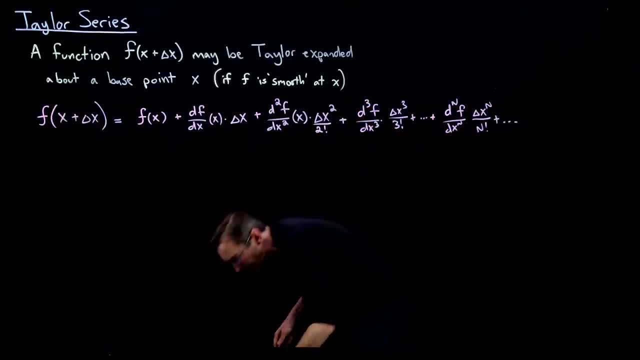 If you want to approximate this, then your delta x better be small. Good, So that's the Taylor series. There are alternate ways of writing this, So sometimes I'll write it like this when we're doing numerical approximations. Sometimes I'm going to write it in the other way, which is, I'll say, or f of x could be expanded. 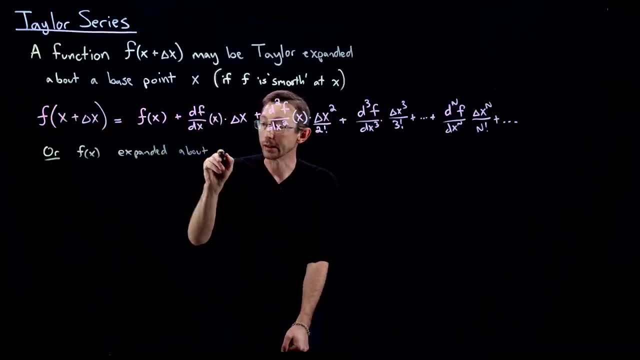 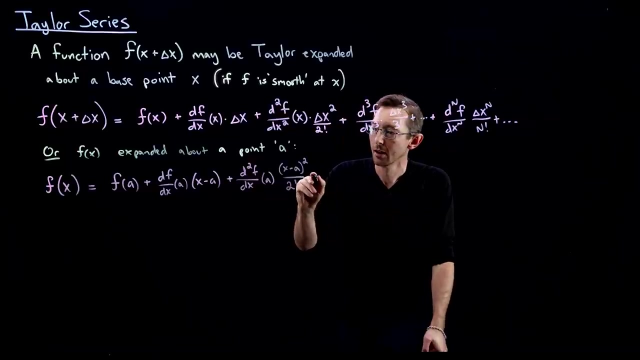 So I'm going to say f of x is going to equal f of a plus my derivative of f with respect to x evaluated at a times x minus a plus, and then I'll talk you through what this means. The second derivative of f with respect to x evaluated at a times x minus a squared over two factorial plus the third derivative, and so on and so forth forever. 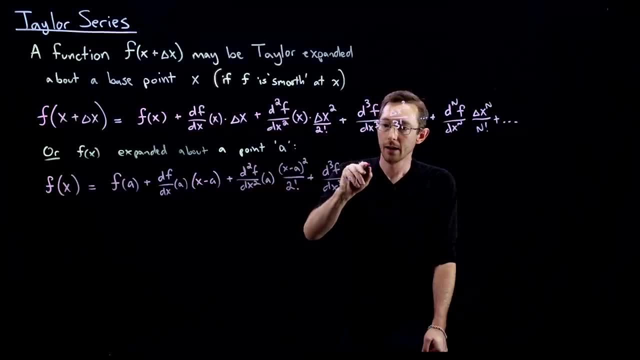 This is x squared, x cubed, x minus a cubed over three factorial plus dot, dot, dot, dot dot. And so essentially what we're saying here, these are just different ways of writing the exact same thing. So if I have, where do I want to write this? 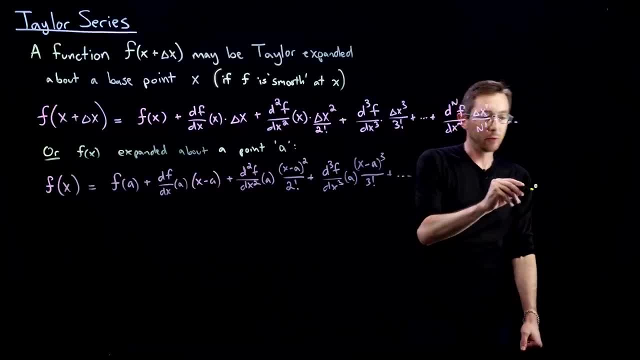 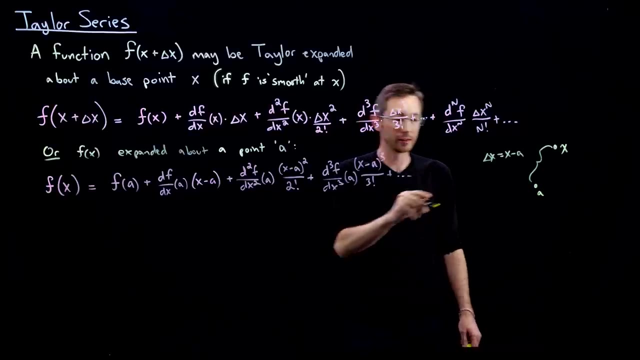 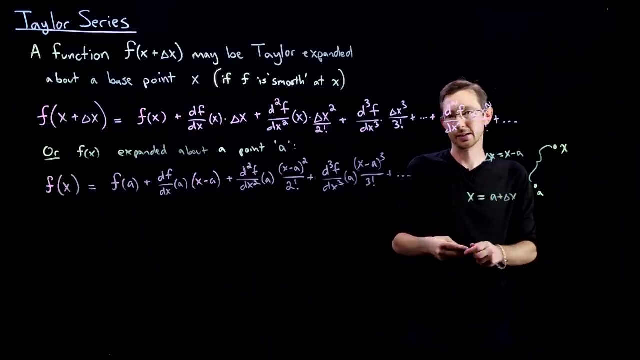 So if I have some point a and I have some point x, then this x minus a is playing the same role as my delta x was up here. So you can just literally say x equals a plus delta x. So this is kind of the exact same expression. 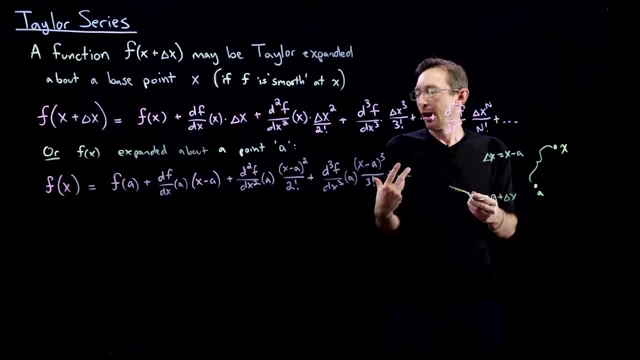 So you can, you can. what am I trying to say? I can pick some point a and then, for any other point, x and whatever x is, I can write down f of x in terms of a and all of its derivatives: A, f of a, f, prime of a, f, double prime of a, f, triple prime of a, and so on. 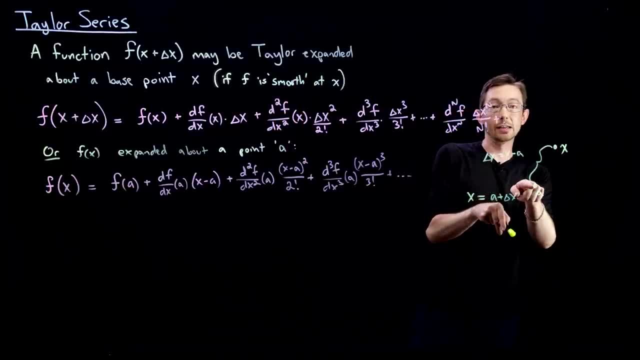 I can write down f of x in terms of just the information I have at this point, as long as my function is smooth. Or if I like to think of this as a small perturbation, a small delta x. I can also think of it that way. 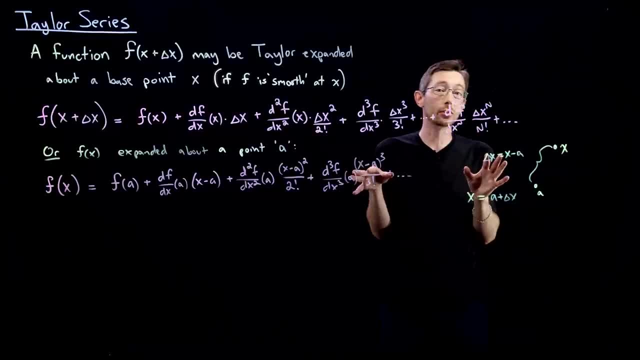 So these are two completely equivalent ways of writing these, and I think this actually would be a good exercise for you is to kind of write these both out and convince yourself that these are in fact identical to each other. if you write down kind of this relationship here: 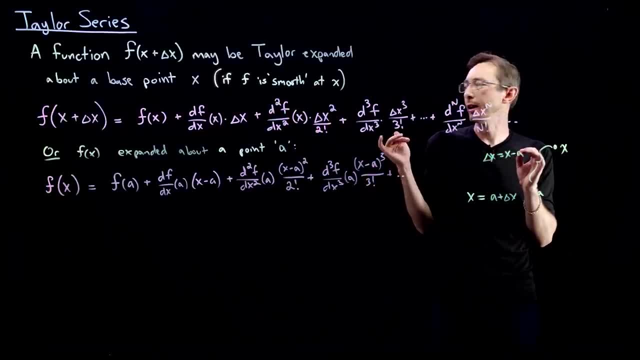 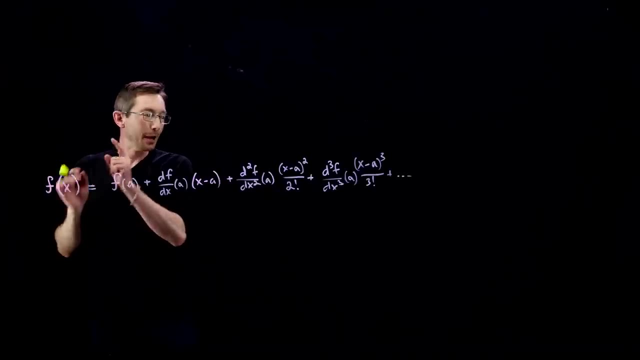 Good. So now what I'm going to do is I'm going to actually do this for an example of a sine function and a cosine function, and then we're going to plot these in Python and MATLAB- Good, Good. So I'm actually going to use this formula for my example of f of x equals sine of x. 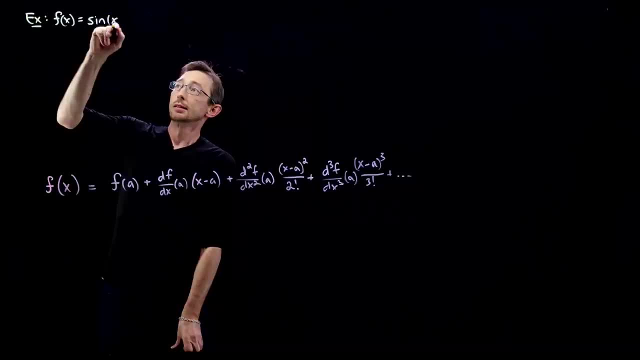 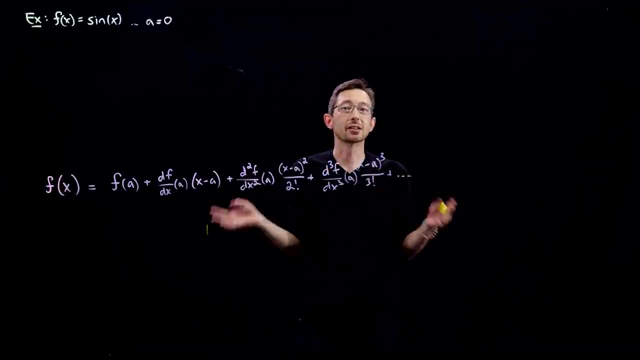 Example f of x equals sine of x and we're going to use the base point. a equals zero. So this is actually a special case of the Taylor series called the Maclaurin series. This is the Maclaurin. how do I spell Maclaurin? 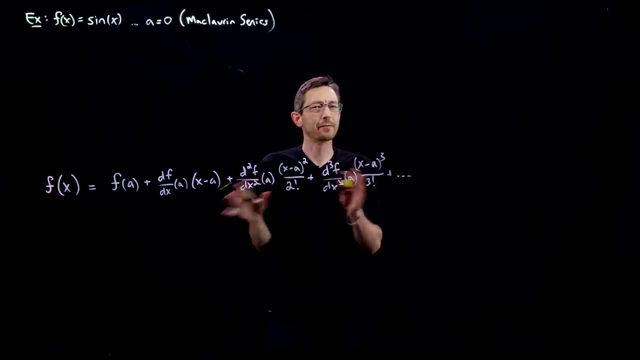 Maclaurin series. If the base point a equals zero- And that's very, very common, because you'll find that it's going to be really easy to evaluate these derivatives at a equals zero- okay, So we can literally write this down. 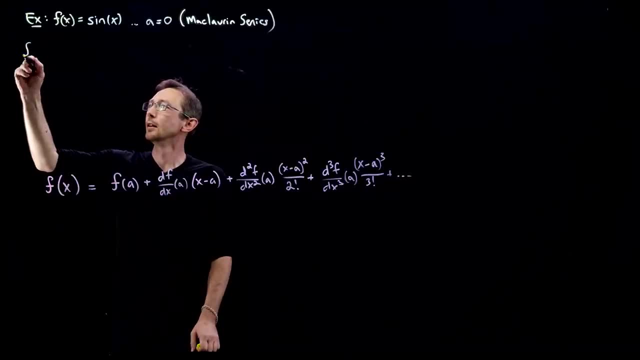 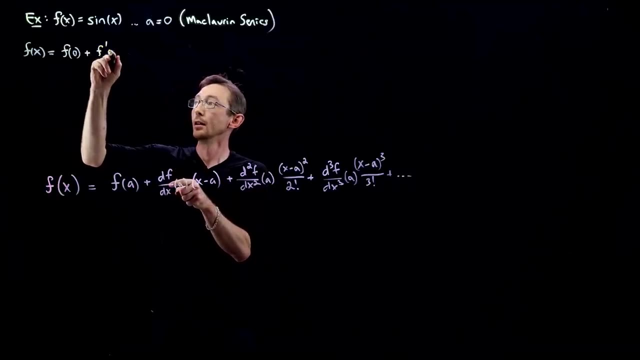 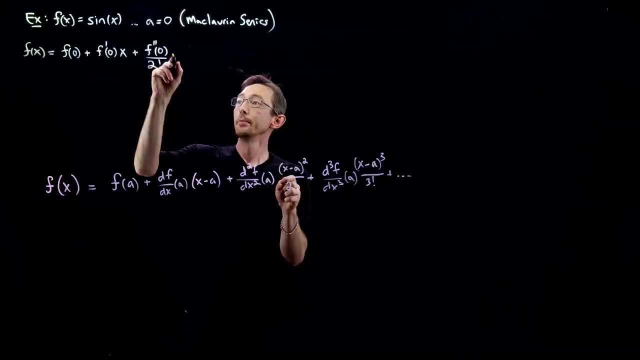 This is super easy: f of x is going to equal f of zero plus f prime of zero times x. And again x minus a when a is zero is really easy. So that's f prime at zero times x plus f Double prime at zero divided by two factorial times x squared, plus f triple prime at zero divided by three factorial x cubed. 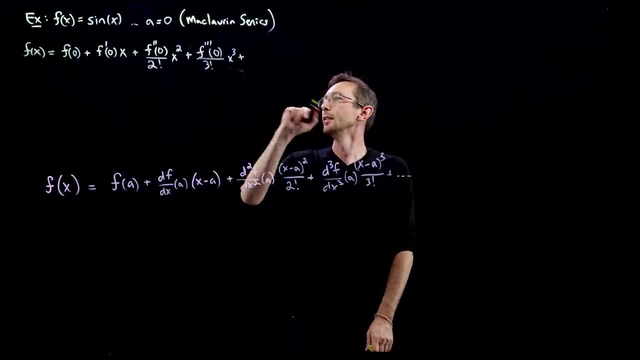 And how many do I want to write? I'll probably go up to fifth order, just because this is important to see what happens. The fourth derivative: zero over four factorial x to the fourth power plus the fifth derivative. Sometimes you put these in parentheses, like that: 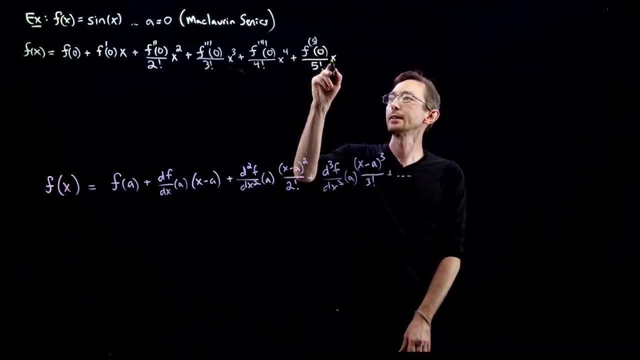 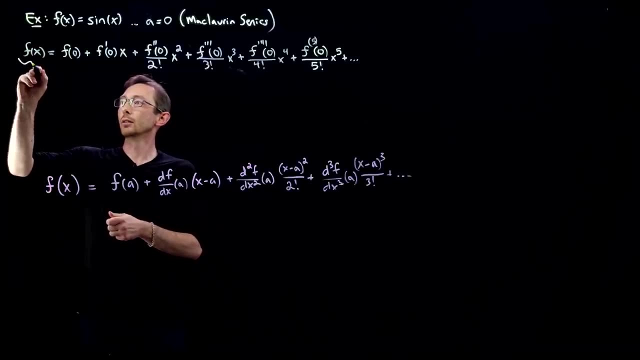 The fifth derivative of f at zero over five factorial X to the fifth, plus dot, dot, dot. This never ends. This goes on forever and ever and ever. This is only exact. This is literally. you know, sine of x is only equal to this. if I add all of these terms up, ad infinitum. 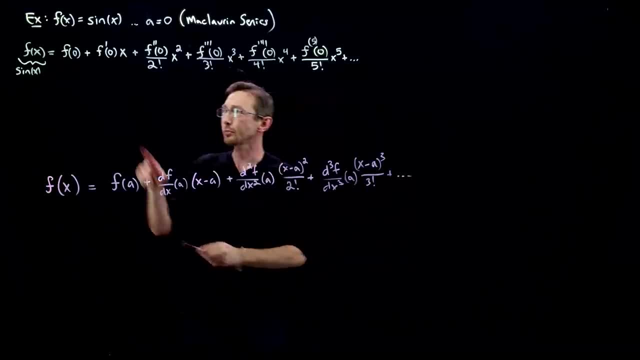 I'm just stopping at five because I can't, you know, I'm not infinite. Okay, good, And so I literally take f of x and evaluate it at zero. So sine of zero. Okay, this is sine of zero plus what's the first derivative of sine. 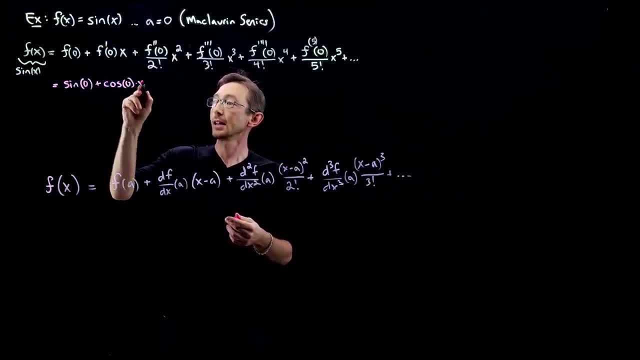 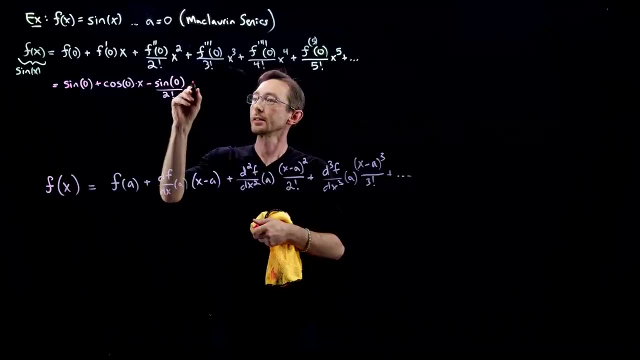 It's cosine. So that's cosine zero times x plus. now what's the second derivative? The derivative of cosine is now minus sine. So this is minus sine evaluated at zero over two factorial x squared. Now the third derivative of sine is minus cosine. 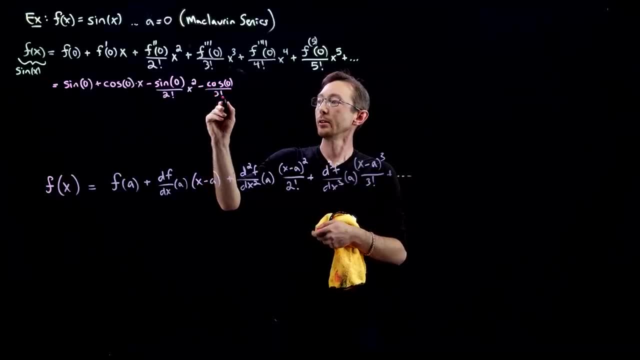 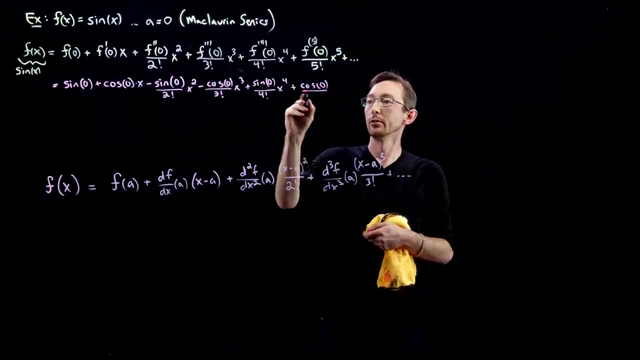 So minus cosine of zero over three factorial, That's a three x cubed. The fourth derivative comes back to a positive Plus sine of zero over four factorial x to the fourth, Plus cosine plus minus. plus cosine of zero over five factorial x to the fifth: plus dot, dot dot. 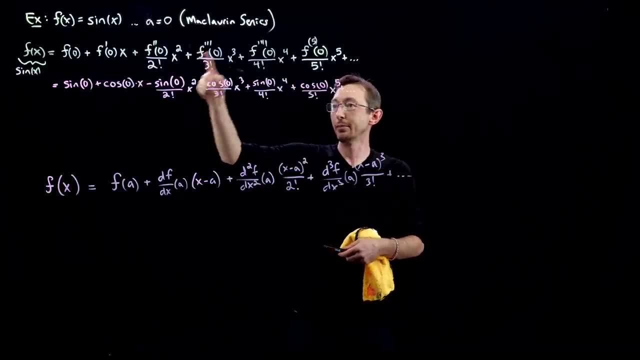 And you see, the pattern is: I have, you know, sines for the even powers And I have cosines for the odd powers. And the sine flips, because when I take the derivative of sine, the first derivative is cosine, The second derivative is negative sine. 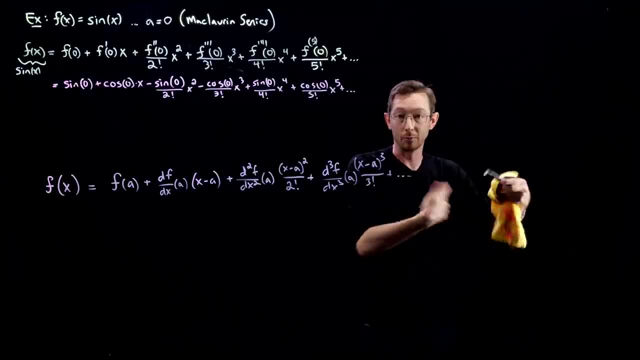 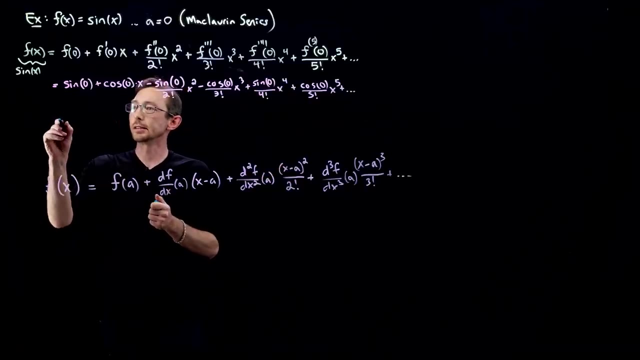 That negative cosine and positive sine, And it repeats every four. Okay, And this is the last step: Evaluating sine of zero and cosine of zero is super easy: Sine of zero is zero, Cosine of zero is one. And so now we find our series: is, you know, zero plus one times x, minus zero, x squared minus you know cos is one? 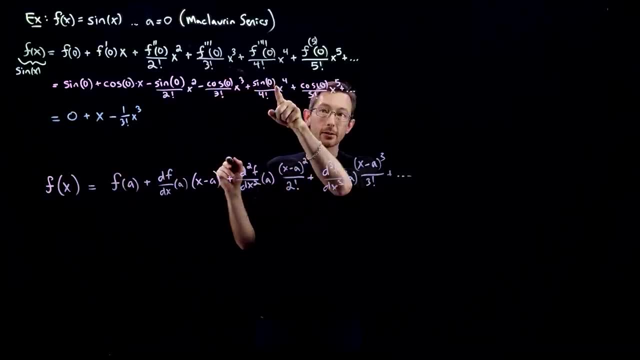 That's one over three. factorial x cubed. plus sine of zero is zero, So I don't have any even terms. Plus cosine of zero is one, One over five. factorial x to the fifth: dot, dot, dot, dot, dot. you know plus forever. 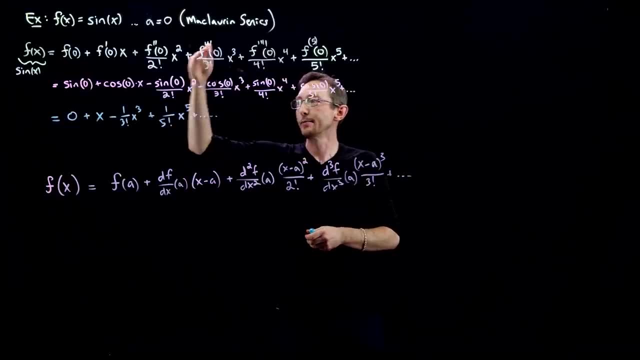 So what you see here is all of the even powers of x are zero because sine of zero is zero. And I only get these odd powers because cosine of zero is one And the sine will alternate. So I can even write this down. You know, I know this is going to be x minus x, cubed over three factorial plus x to the fifth over. 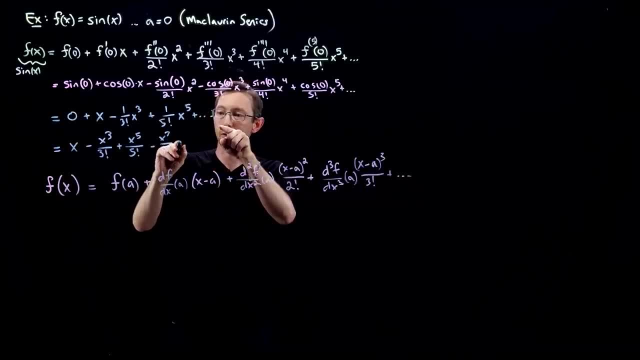 Five factorial minus x to the seventh, over seven factorial plus x to the ninth. I know the pattern, So I can keep doing this forever and ever. And this is my Taylor series expansion, Or technically my McLaurin expansion for sine of x. 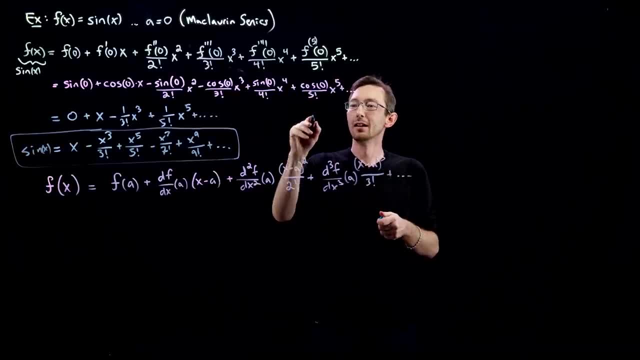 And it is odd. So this is actually really comforting because we know that the sine function. if I actually literally draw sine of x, it is an odd function like that Meaning. you know it has this kind of mirror symmetry. If I take sine of minus x, it is minus sine of x. 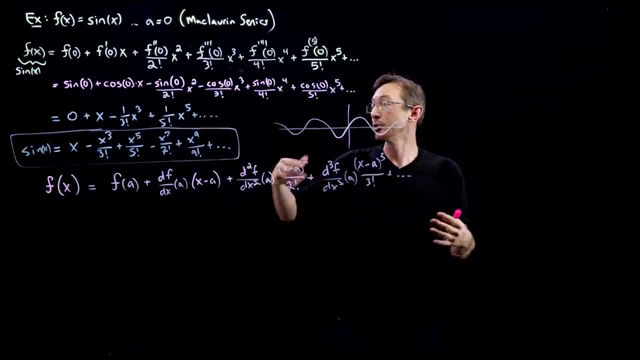 And so I can only achieve that with these odd powers. It's literally an odd function. So it's cool and reassuring that the Taylor series- all of the odd terms- are the only ones that stick around. Good, Okay, that's sine. 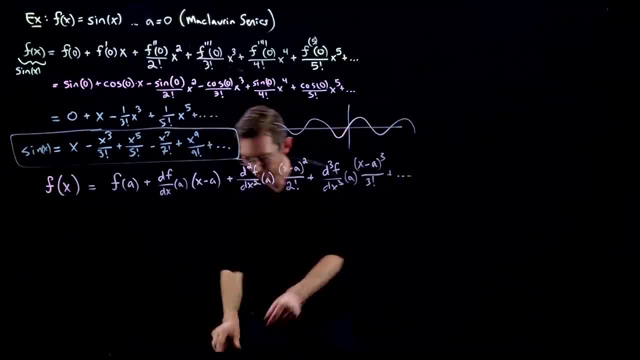 I'm going to do the same thing for cosine, And then I'm going to do Python and MATLAB. Okay, So let's do the same thing now for cosine. So example: What is f Of Of x equals cos x when I McLaurin expand it. 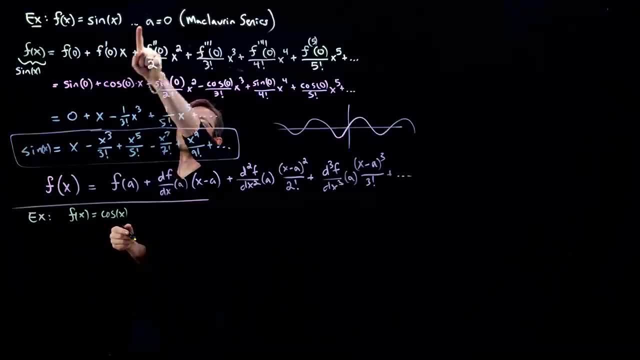 Same exact thing. It's going to be f zero plus f prime zero, x plus f double prime zero over two factorial x squared, and so on. And so I'm going to get you know: cosine x equals cosine of zero, Plus the derivative of cosine at zero is, you know, minus sine of zero. 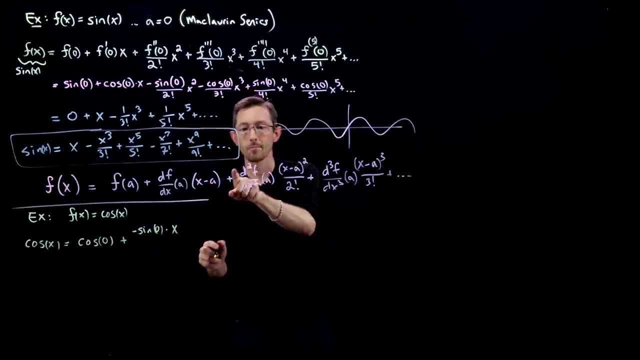 Times x, plus the second derivative of cosine at zero, which is again minus cosine zero divided by two factorial times x squared, plus the third derivative of cosine, which I believe is now going to be a plus sign, plus sine of zero over three factorial x cubed, plus the fourth derivative, which is plus cosine of zero over four factorial x to the power of zero. 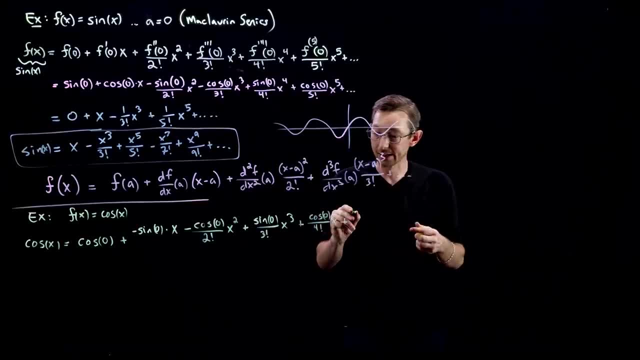 Plus. now the fifth derivative is again a minus sine zero over five factorial x to the fifth minus, And I'm just I'm writing this down because you can almost intuit what the answer is going to be, from the pattern minus cos of zero over six factorial x to the sixth plus, dot, dot, dot, dot dot, forever and ever and ever. 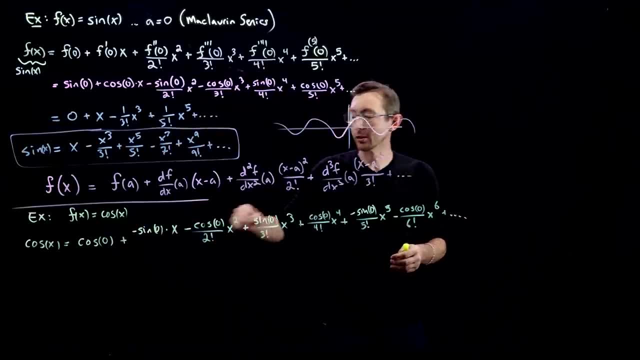 And so, again, the only terms here, all of now the odd terms- are going to be zero, because those are the ones that have signs. So sine of zero is always zero. So Zero, zero, zero. And the only terms left are these ones that have a cosine of zero, because cosine of zero is one. 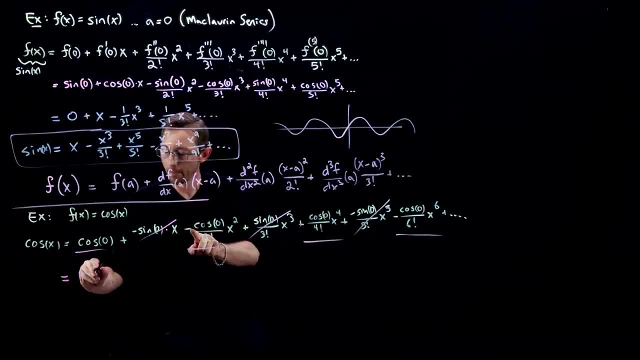 And so this equals now one minus one over two factorial x squared, plus one over four factorial x to the fourth, minus one over six factorial x to the sixth, And of course you can just write this down forever And ever: one over eight. factorial x to the eighth, plus dot, dot, dot, dot dot. 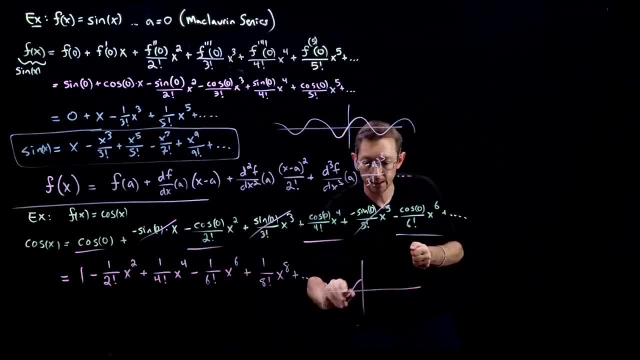 And again, because cosine is an even function, Meaning that cosine of negative x equals cosine of x. I can only achieve this with the even powers in the Taylor series expansion. So this is just a double check of our intuition. because cosines an even function. 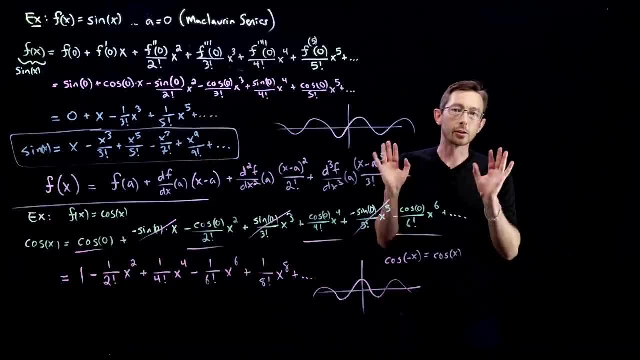 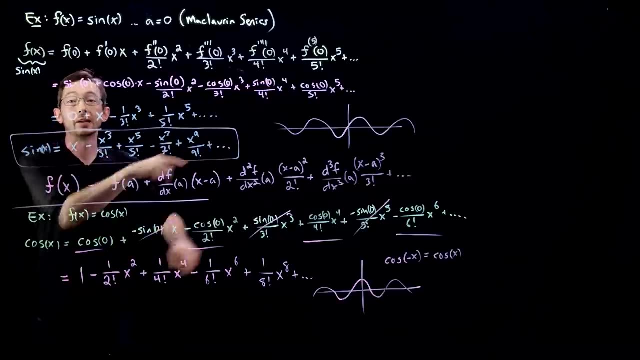 It can only have these, even powers of x. OK, good, So really easy to compute the Taylor series or the McLaurin series For Our functions, that we are interested in, that we know and love. You'll notice that the sine and the cosine terms almost have all of the terms from the exponential e to the x. 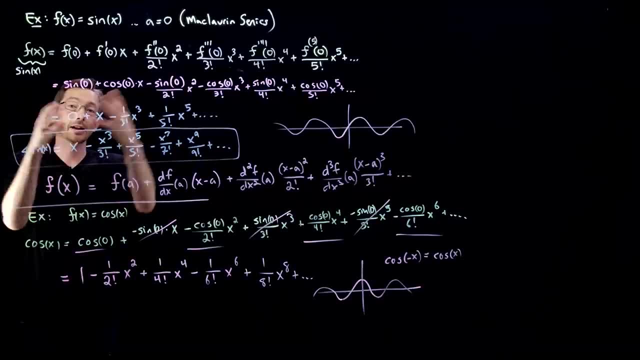 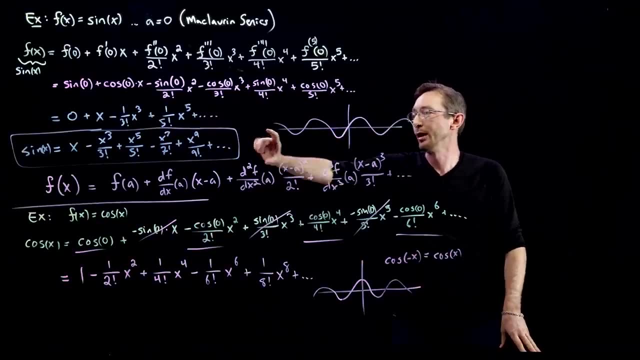 And so we'll show in the next lecture that if you take, you know, e to the x, you can actually break it down into its sine components and its cosine components. That's very important. That's called Euler's formula. But for now I'm just going to pick this sine of x expression, and we're actually going to plot this in MATLAB. 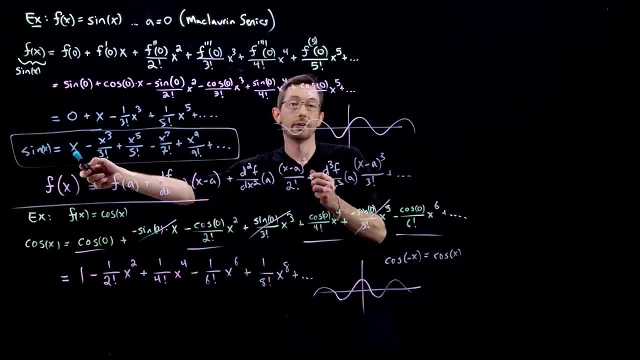 We're going and Python, We're literally going to show that if I only Have the first order approximation, it'll be this linear approximation And then if I add the next term, this cubic, I'll get a slightly, I'll get a slightly better cubic approximation. 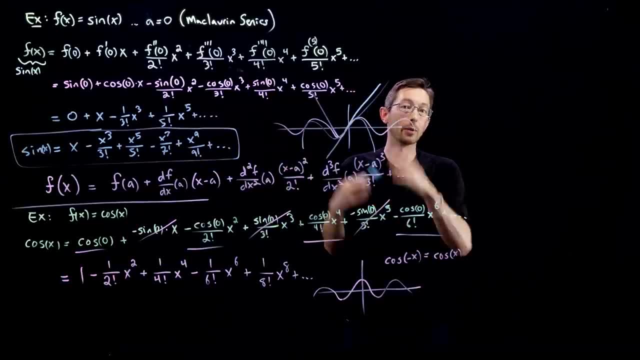 And when I add the fifth, I'll get a slightly better fifth approximation And we'll just add this up and show that this really does approximate my function. as I add more and more terms, I mean I erase this and then that's what we're going to do. 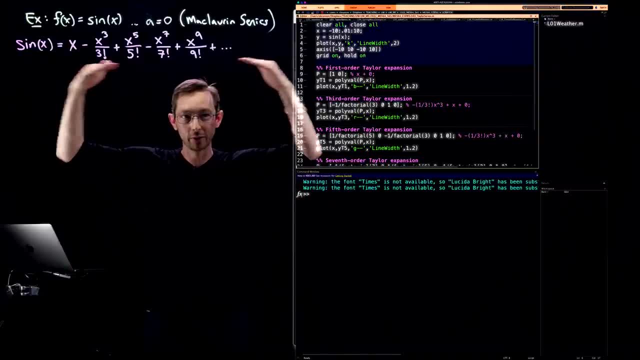 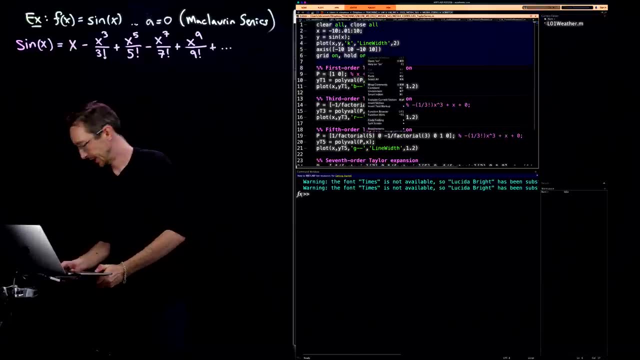 OK, So I move my equation up here, So I have a little bit of breathing room, and I'm going to do this in MATLAB and in Python, So I think I'm just going to start with MATLAB. This is the code I wrote, probably 10 plus years ago, to demonstrate this concept. 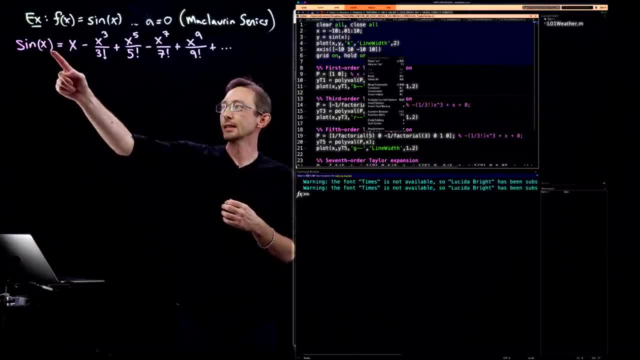 OK, So essentially, what I'm going to do is I'm literally going to approximate sine of x using the first order term, the linear term, x, the cubic term, x, cube, the fifth order quintic term, the septic term, the nonic term. 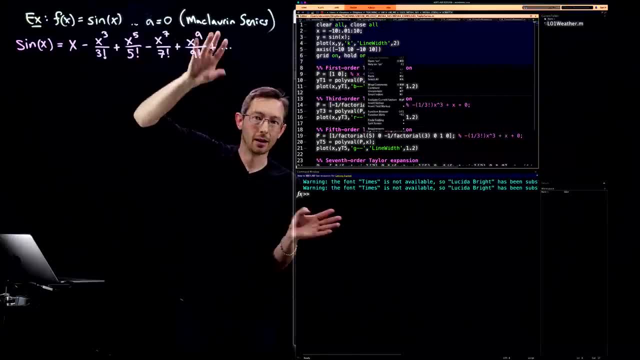 I think those are cool names: Cubic, quintic, septic, Nonic. I don't know what's after that. If you do, please tell me. And so, essentially, I'm just going to walk you through this code, I'm not going to write it from scratch. 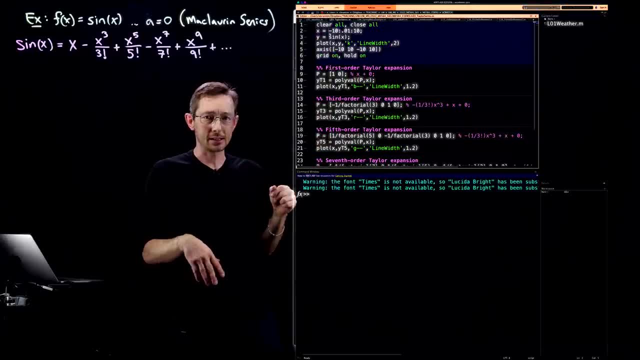 You can download this, The first block of code here, from lines one to six. all it does is it just plots my function, my sine function, from x equals negative 10 to x equals plus 10.. And I've called this y, when in reality I really should have called this f of x. 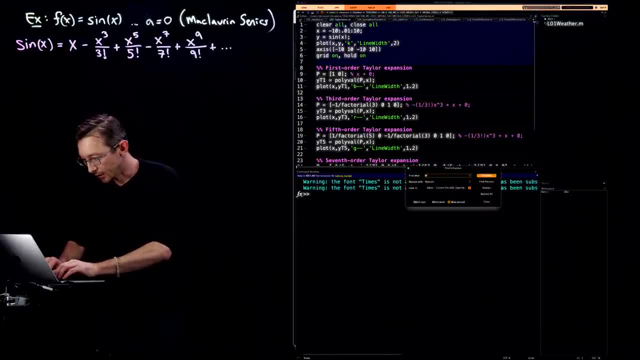 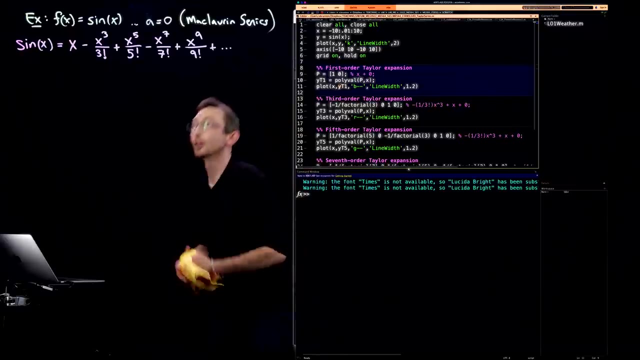 I wonder how many y's I have. I wonder if this is going to butcher everything. if I do, y equals F, let's see, Nope, that's going to mess everything up, OK, well, you all are very bright and you can. you'll be OK with the fact that now we've just renamed this. 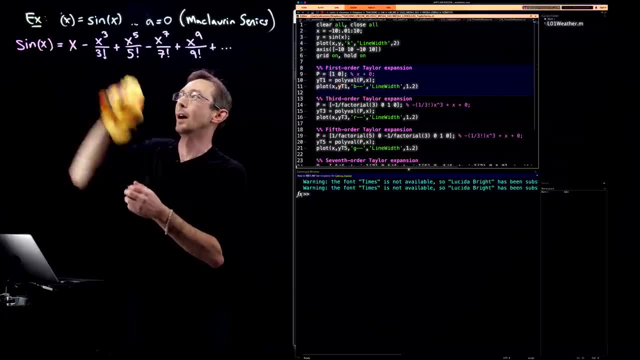 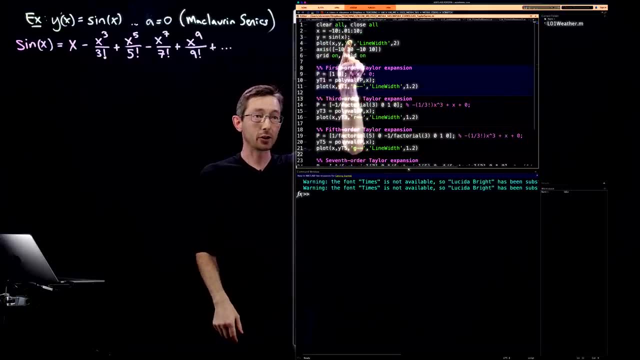 We're calling this y of x. OK, we're calling this y of x. Good, So the first thing I'm going to do is I'm just going to plot my function y of x. That's going to be the ground truth. 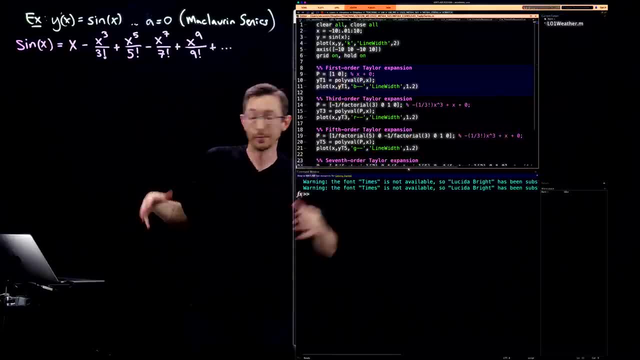 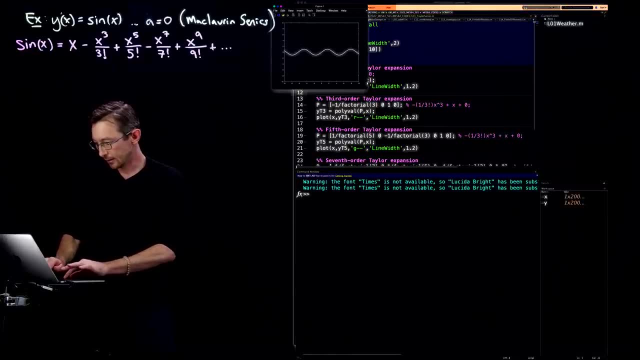 And then we're going to compare the linear, the cubic, the fifth, the seventh, the ninth order approximations. So first things first, let's just run this And I'll make this a little bit bigger. OK, Sorry, my axes are all so small. 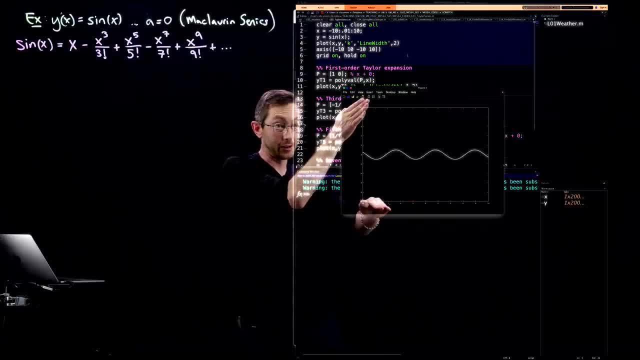 This is, you know, time and this is sorry. this is x and this is y of x, my sine function, And it looks like you would expect it, expect it to look. And now what I'm going to do is I'm going to compute my first order. Taylor series- approximation. 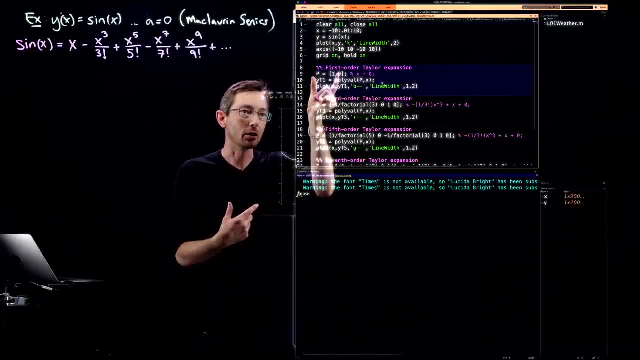 Which the way you do this in MATLAB is, you can create a polynomial. This basically p equals one zero means that you have a polynomial one in the x to the one and zero in the x to the zero. So it's literally x plus zero and polyval of p. comma x evaluates that polynomial with those coefficients on this data vector x. 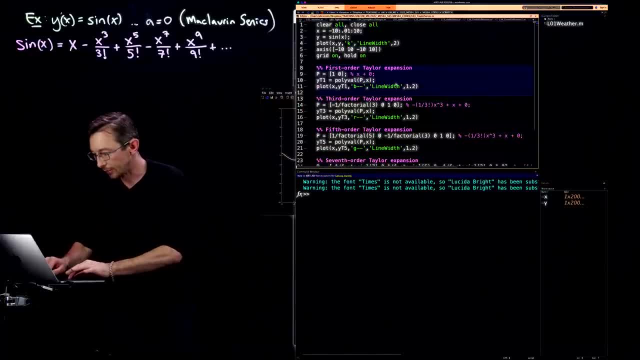 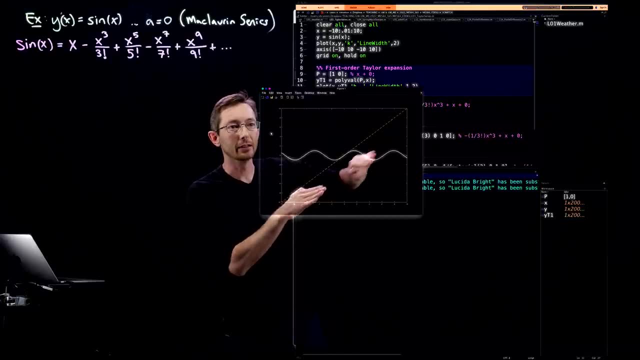 And that returns my fit y. So here now I can plot this one On top of it And you can see this is literally my linear fit, my, just the first term, my first polynomial approximation, And it's actually not terrible- Like it's obviously terrible out here, but it's not so terrible for a small region around the origin, for a small x near zero. 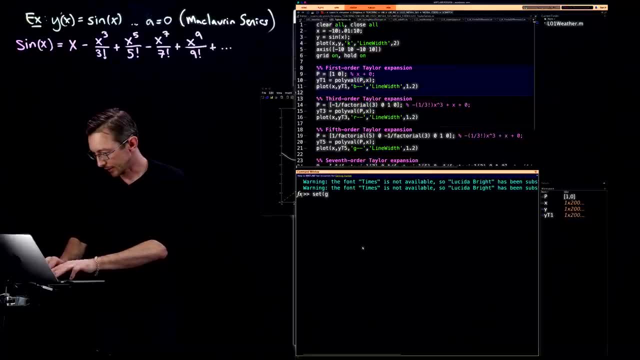 It's not too bad. Maybe I can make my set GCF font size 14.. Does that make it better? Nope, GCA Font size. There you go, Let's make it 24, just to make everything a little easier. 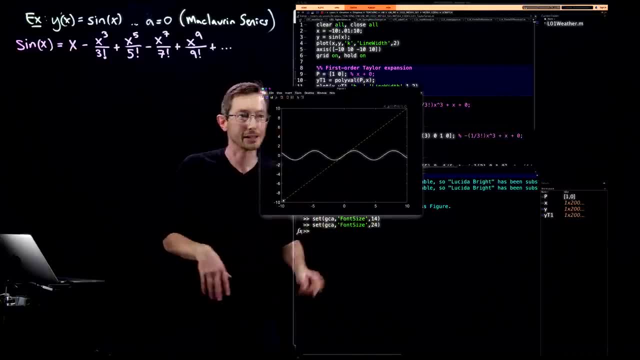 Okay, I should have done this easier. Now you can see all of the plot axes. It starts at: x equals zero. This thing looks pretty good, But what happens when I do a higher order polynomial? So now what we're going to do is we're going to do a third order. Taylor series- approximation. 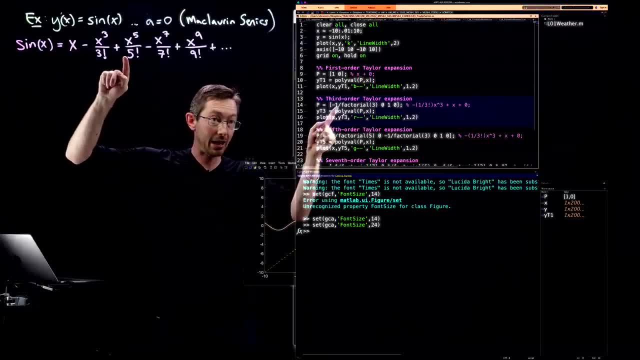 So again that polynomial has coefficients and it goes in order from biggest power to smallest power. So this one should have a minus One over three: factorial in the x, cubed, a zero in the x, squared, a one in the x and a zero in the ones. 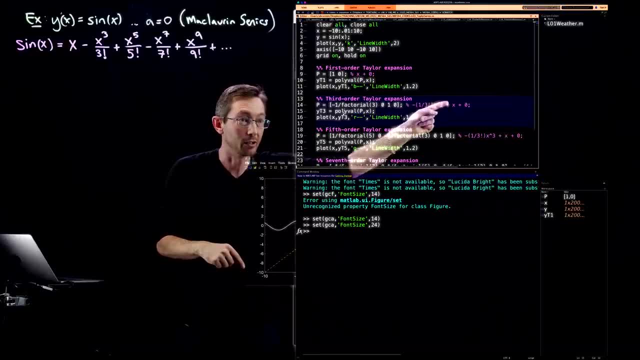 This is literally one minus one third, one over three factorial x cubed plus x plus zero. I'm going to evaluate my polynomial with polyval on x and I'm going to plot this y Taylor series three. Let's see if that works. 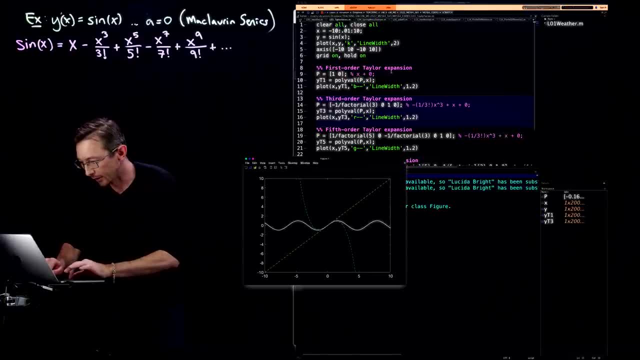 Okay, And now you can see, maybe I'll make all of my line widths 11.5.. A little bit bigger, So I'll make these. you know, I'll make this one like five and I'll make all of my. 1.2 is equal to two. 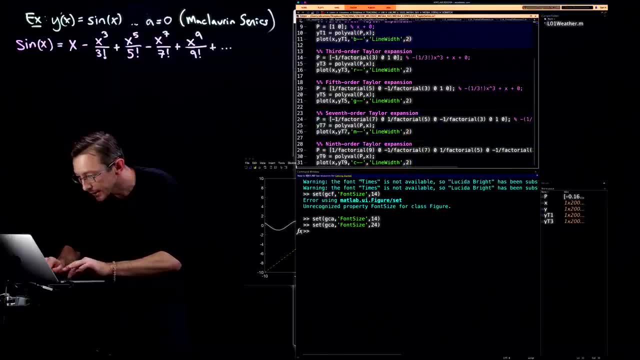 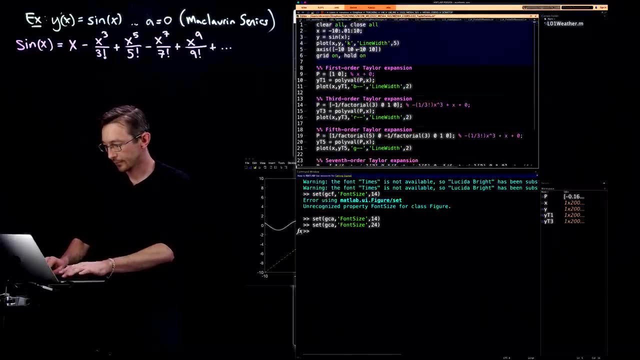 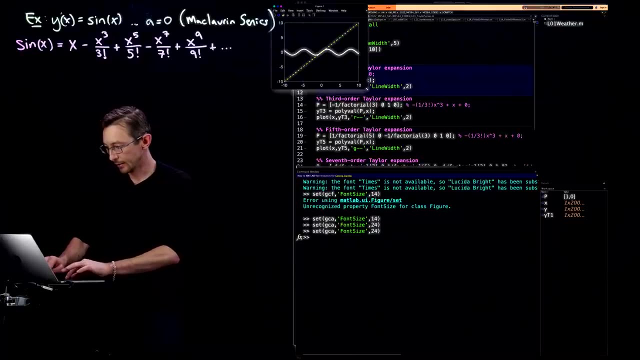 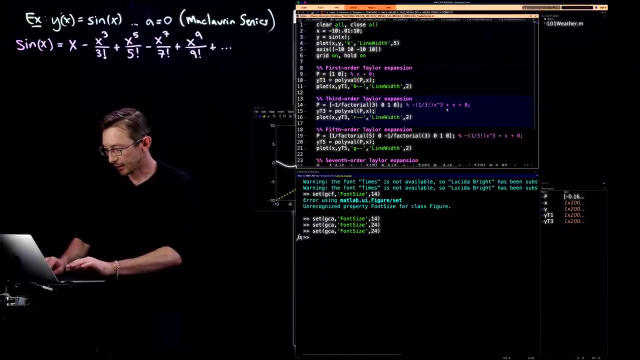 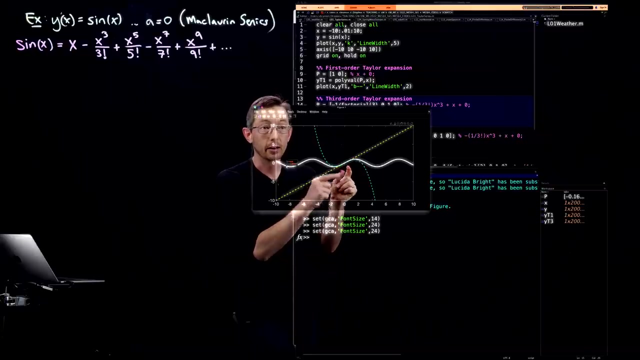 Replace, replace, replace, replace. This will be a little nicer. Make my font size big again. Okay, good, So now everything is a little bit cleaner. I have my third order polynomial here and you can see that again. for small x, for x near zero, it's actually really good and it's slightly better than linear. 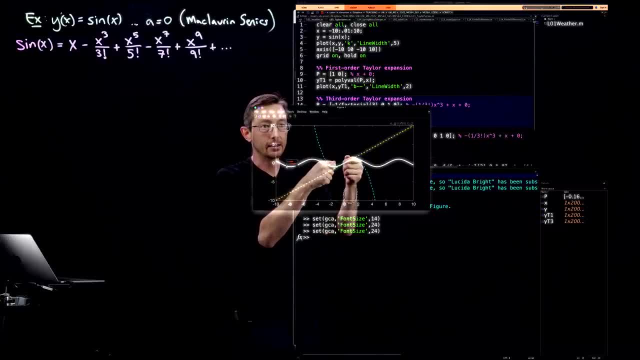 So it's very hard for me to do this mirrored, but you can see that it's actually getting a little bit better of an approximation of that first term in the sine function. So the cubic approximation is a little bit better than linear, And then, similarly, I can add a fifth order, polynomial. 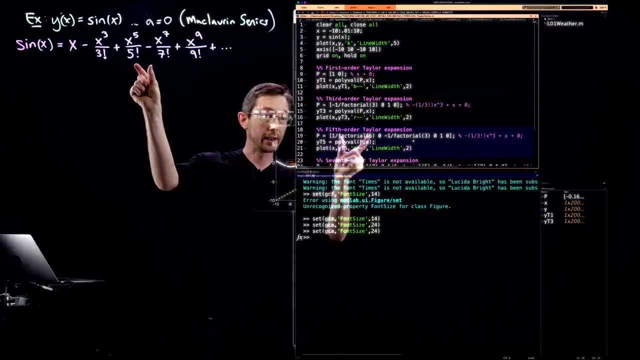 Now I'm just making a bigger polynomial that has this fifth order term, So that's one over factorial five in the x to the fifth place, zero in the x to the fourth, and so on and so forth. So this is my fifth order polynomial. 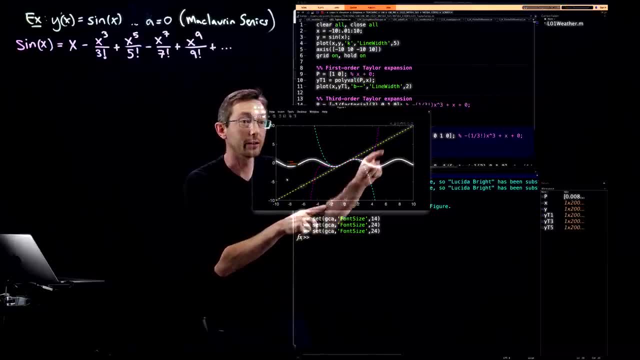 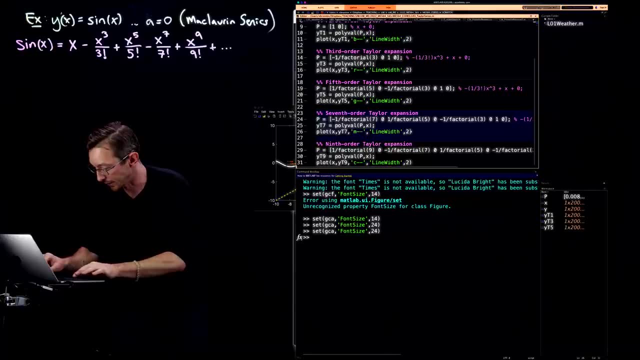 Again in purple. now you know, my fifth order polynomial is doing even better. It's capturing even more of these kind of bends or camel humps, And I think in this script I go up to ninth order. So I'll just actually do all of that and then I'll pop in. 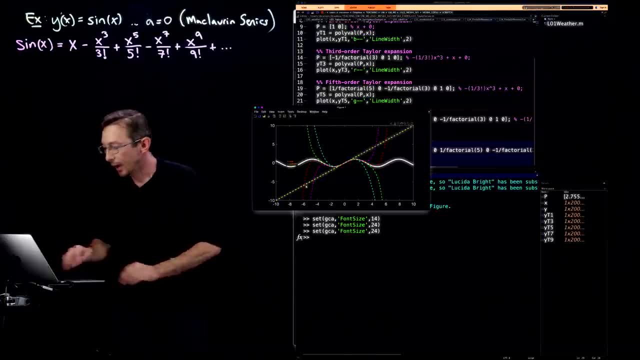 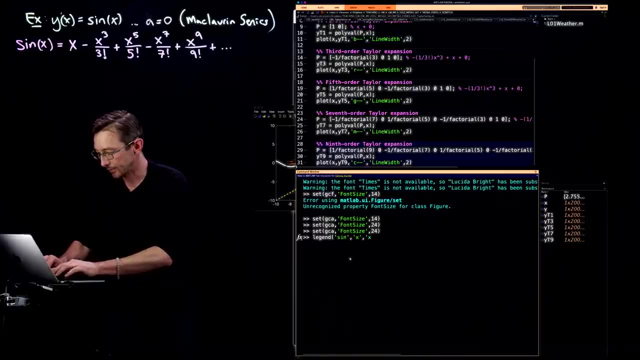 Do I have a legend? I seem to be completely missing a legend here, But you can see, Let's just do legend. Legend sine x, you know, x cubed, cubic, quintic, septic and nonic. 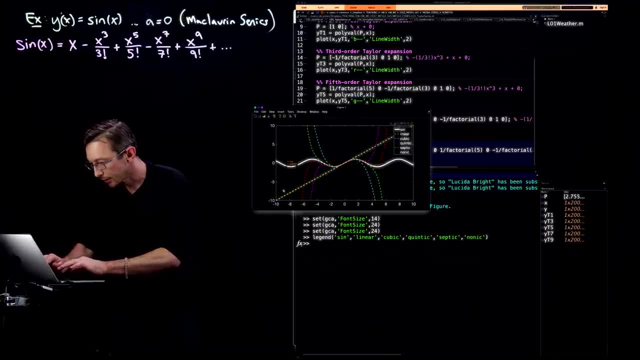 And maybe I'll call x linear. Is that going to work? That's going to work, Okay, so this is kind of the outcome. So you see that every term that you include gets better and better and better. It kind of expands this radius of how accurate your Taylor series approximation is. 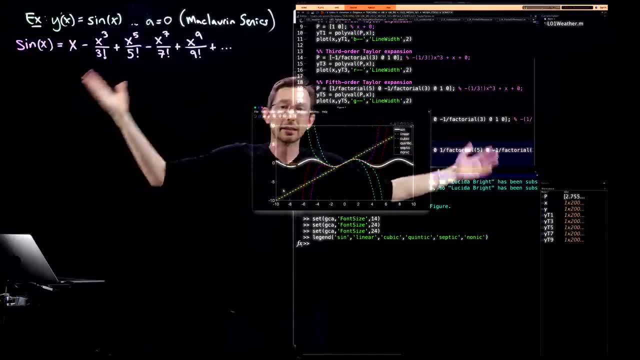 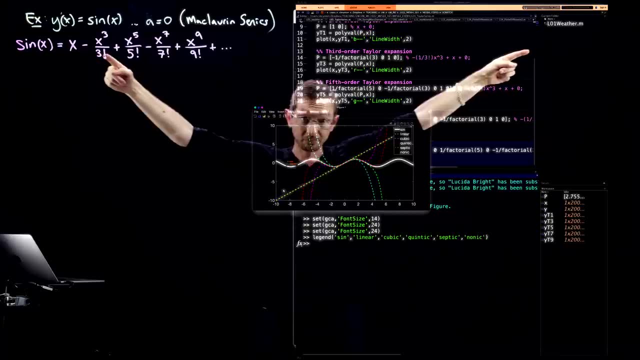 Now, clearly, you know, at very, very far distances, polynomials are a terrible approximation to sine. You know out: at: x equals 100 and x equals minus 100, I would need a huge amount of this series to fit that function. 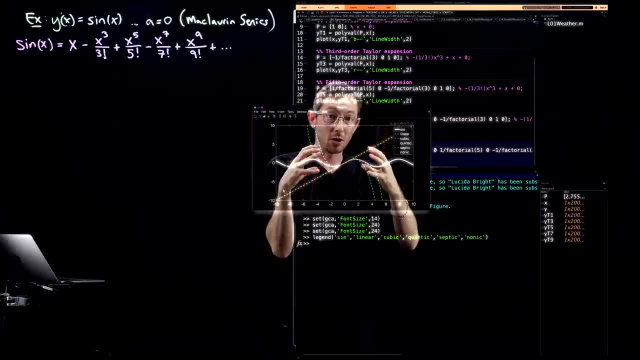 you know, for very, very large x, but at least for a reasonably small x, this is getting better and better and more and more accurate. So this really does do a good job of approximating these functions through this Taylor series approximation. Okay, if you really wanted to approximate a sine function, you should use a Fourier transform. 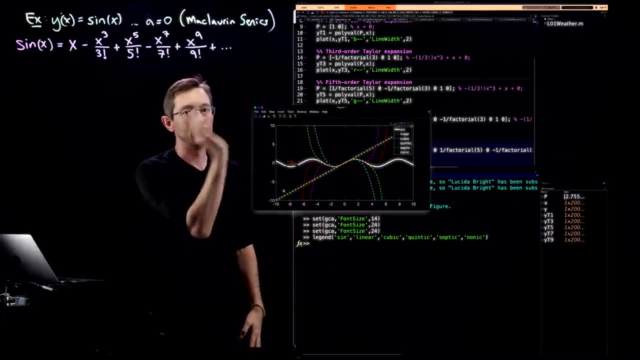 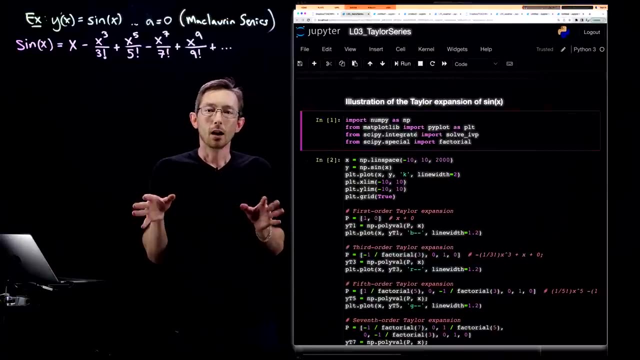 Not a Taylor series. You should use a Fourier series and that'll be a whole, you know- set of lectures later on. Good, Okay, now I'm just going to swap this out and do the same thing in Python. Okay, so we are trying to show that this Taylor series, technically it's a Maclaurin series. 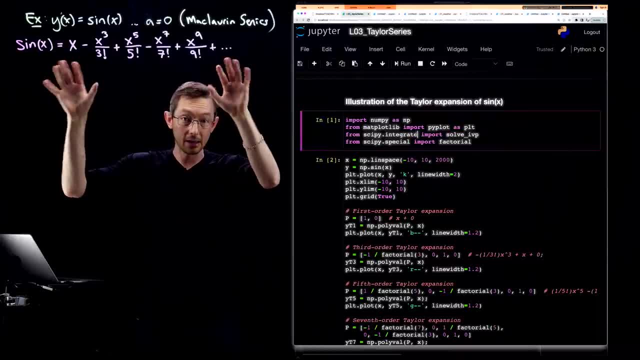 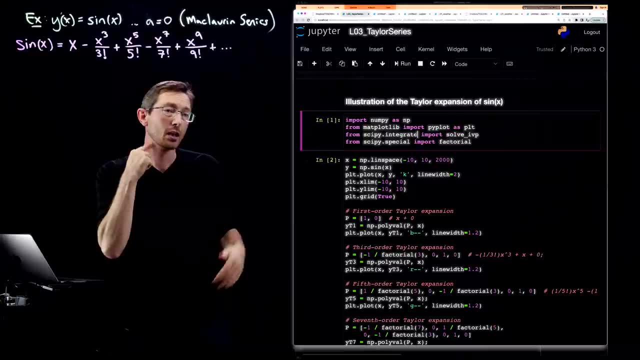 because it's based at zero. this series approximation for sine of x in terms of polynomials actually does an increasingly good job of approximating that function. So this is a code written by Alan Captainoglou based on one of my MATLAB codes. This is in Python, and so I'm just going to walk you through. 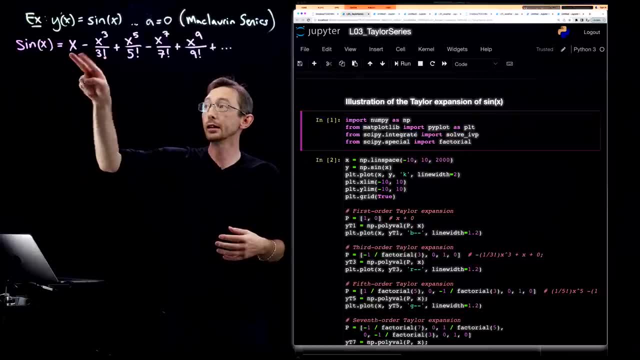 what happens if we only use the linear approximation for sine, or only the linear plus cubic, or linear plus cubic plus quintic, And in this case we have our linear, cubic, quintic, septic and nonic terms. So you know. but you can go higher and higher. 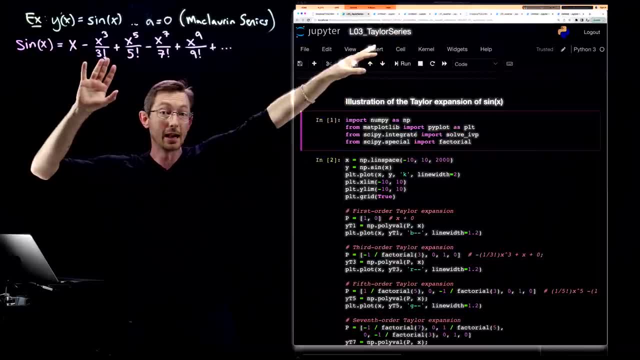 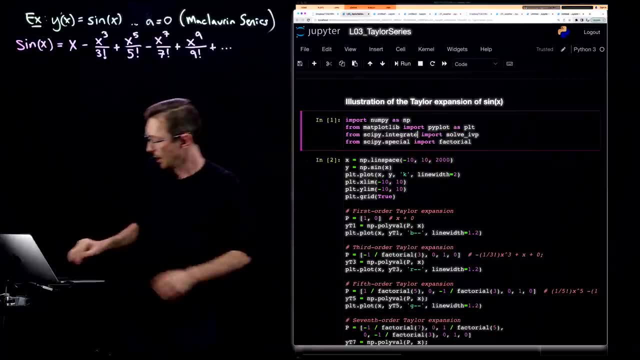 You can add 11th and 13th and 15th and 17th terms- as high as you like, and what we're going to show is that this approximation gets better and better the more terms you add. Okay, so to do this in Python, you have to import some stuff early on. 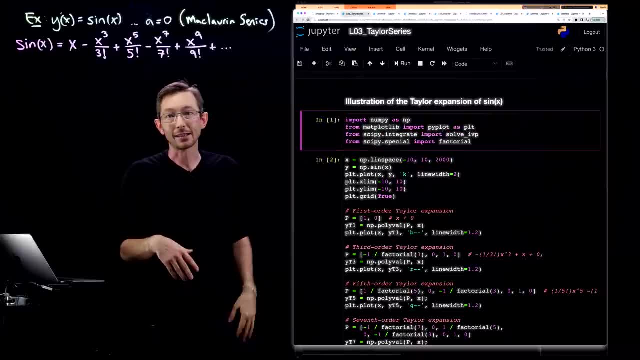 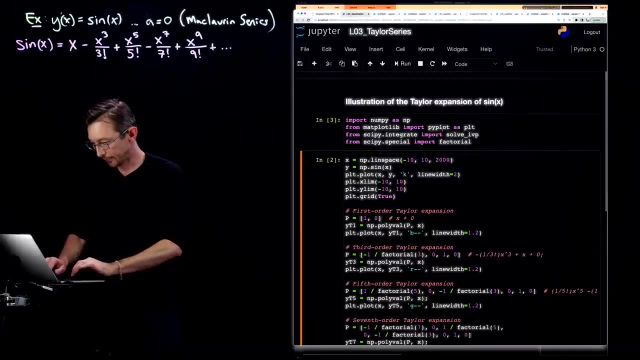 You have to import numpy and matplotlib and things like that, this factorial function, so you can do factorials, so let's do that, And then this is essentially what this code is doing. The first block here is just creating our sine function. 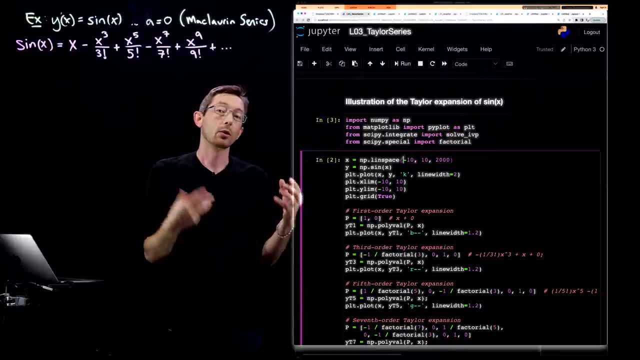 So we're saying: y of x equals sine of x, and that's going to be the ground truth. We're going to compute sine of x on a domain x equals minus 10 to 10, and we're going to plot it and: 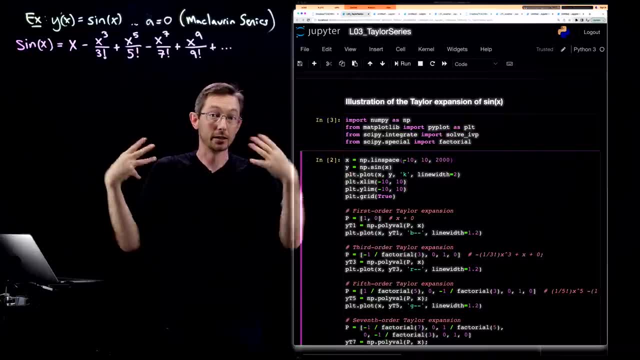 then we're going to plot the linear, the cubic, the quintic on top of that to see if they get better and better and better. Okay, so the first order: Taylor expansion. Essentially, what we're going to do is we're going to define the coefficients of our polynomial 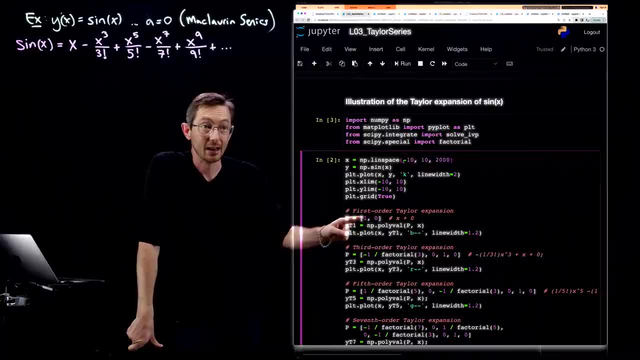 so this goes from biggest term to smallest term. This is the x to the 1 power and x to the 0 power. so this p equals 1, 0. literally means I have 1 of x plus 0 of x to the 0 of 1, and then 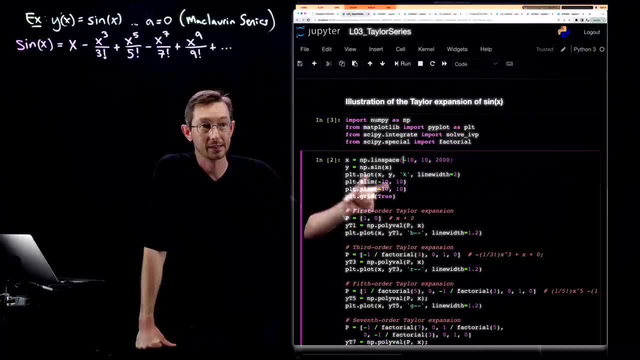 I'm going to evaluate that polynomial on this kind of x vector. So x is a you know a bunch of points from negative 10 to 10, and I'm going to evaluate my polynomial on that vector to get my linear fit which is in this variable yt1, and we're going to plot it. 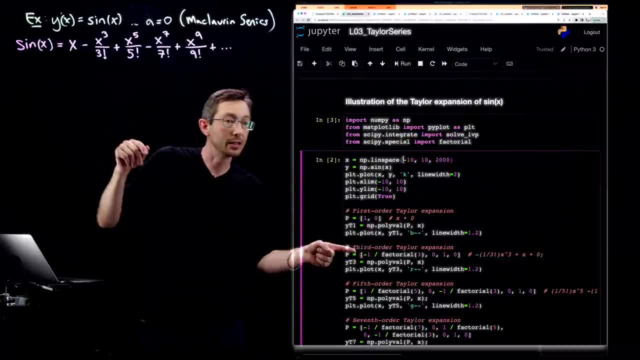 Similarly, we're going to do our third order, Taylor series approximation, which is going to be again. this polynomial is: minus 1 over 3, factorial in the x to the 3 spot, plus 0 in the x squared spot, plus 1 in the x to the 1 spot, plus 0 in the x to the 0 spot. 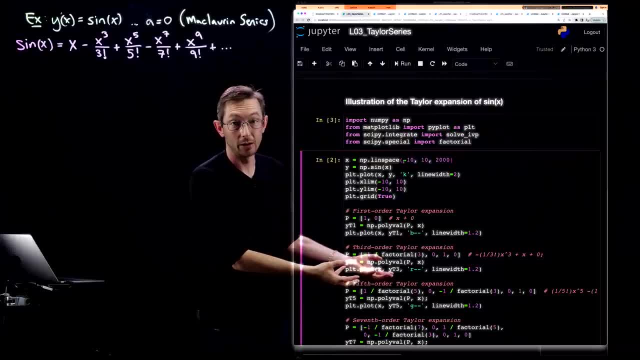 That's this polynomial. We're going to evaluate that polynomial on our data x to get this yt3, which is my third order, Taylor series approximation, my cubic. We're going to plot that and we're going to do that for 5th, for 7th and for 9th order. 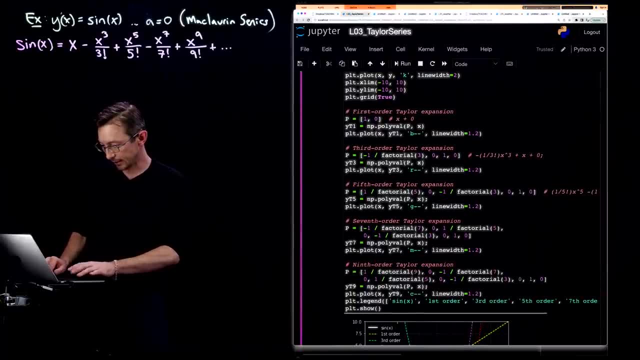 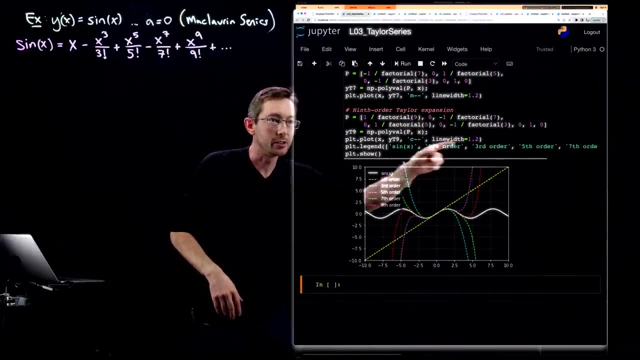 And so if I do this, and then we're gonna, we're gonna plot it. So let's see if I can do this. and Alan added in these legends here, sine of x, first order, second order, third order, fifth order, seventh order, and so on. 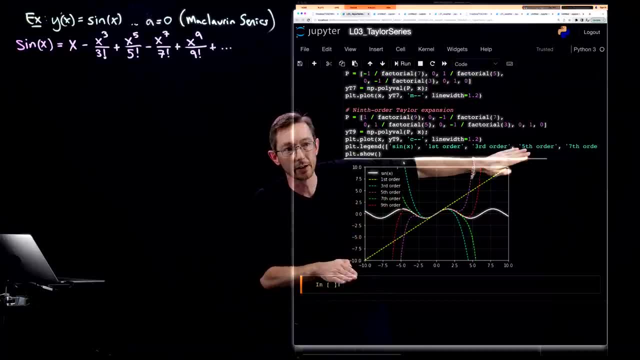 And so you can see. so this, this yellow curve here, is our linear fit and it's actually not terrible. So you know, very close to the origin to, x equals 0. It's actually not that bad, but for far away, you know, very quickly it stops. 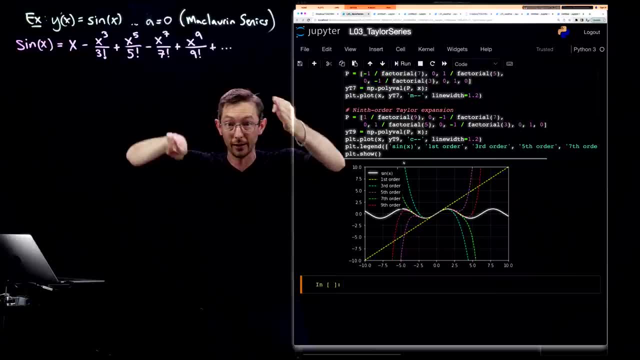 It doesn't capture, for example, when sine turns over, when it kind of, you know, switches directions, and my cubic function, which I believe is this kind of light, blue, cyan one, the cubic function is doing a little bit better. 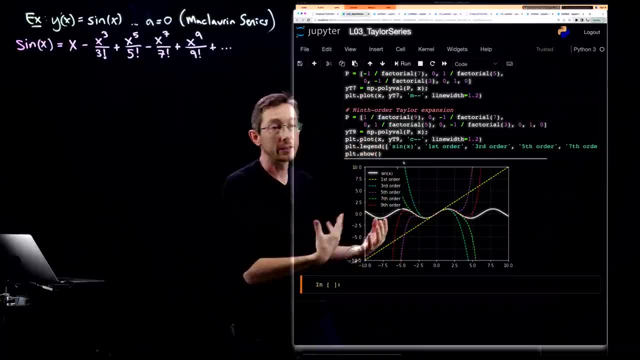 It's starting to capture when sine kind of turns around. The fifth order function in purple here does even better still. And then every term you add, when you add the seventh and the ninth and so on and so forth, it gets a little bit better and a little bit more of that function. 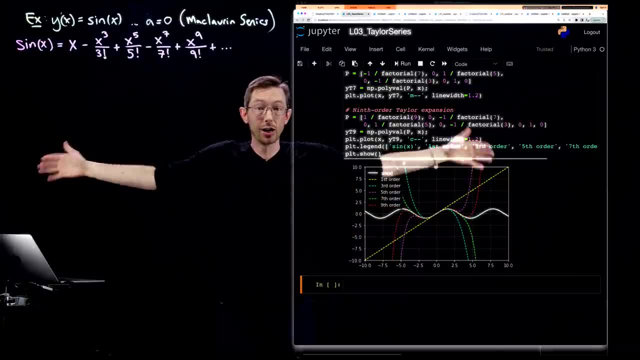 Now, clearly this is going to do a pretty poor job for a very, very large x. You know x equals positive 100 or negative 100.. I'm gonna need a ton of terms in this Taylor series to do a good job. 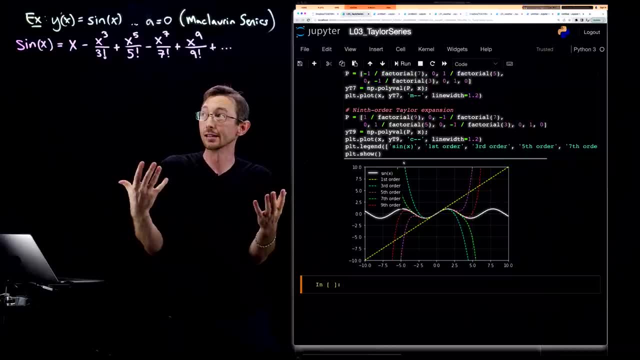 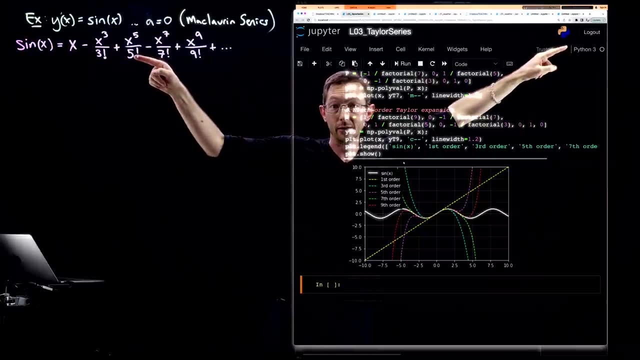 But the cool thing about this math, this kind of calculus, is because this is a smooth function and all of the derivatives exist. if I really did add up all of these infinitely many polynomials, it actually would perfectly approximate sine of x at any point. x I like, even very, very far away okay. 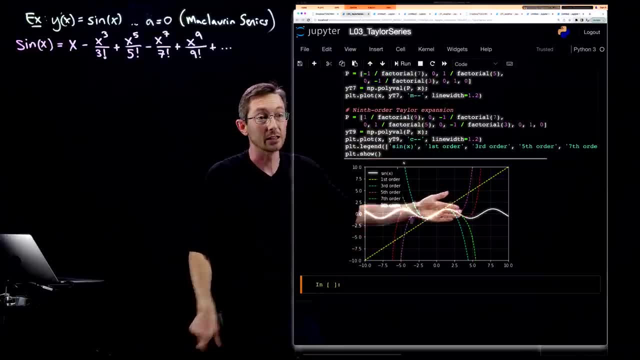 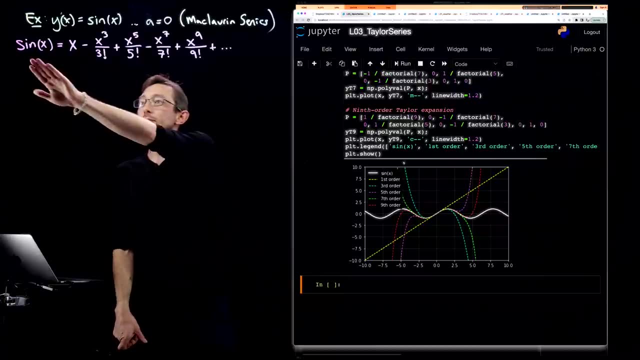 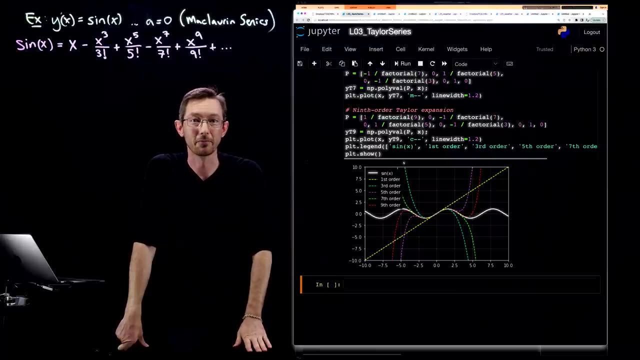 But for numerical approximation, you can see that adding more terms actually does kind of improve the accuracy and the fidelity for a growing radius. okay, Good, and of course we're using these to solve and approximate differential equations. I think that's all I wanted to show you today, so stay tuned for the next lecture, thank you.